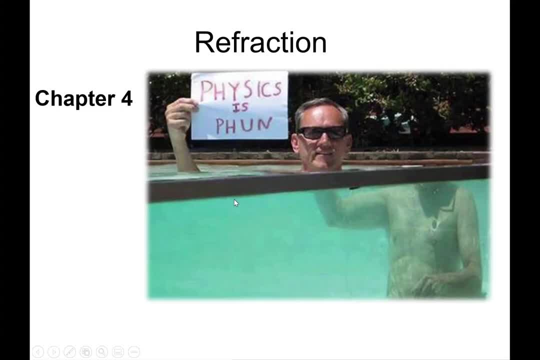 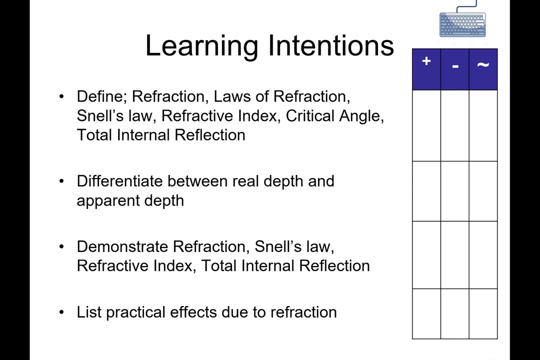 Hello and welcome to this leave and start physics video. Today we are going to discuss the topic of refraction, which I hope you can see from this picture is pretty obvious. Okay, so some of our learning intentions that we need to achieve in order to have a good understanding of this chapter. 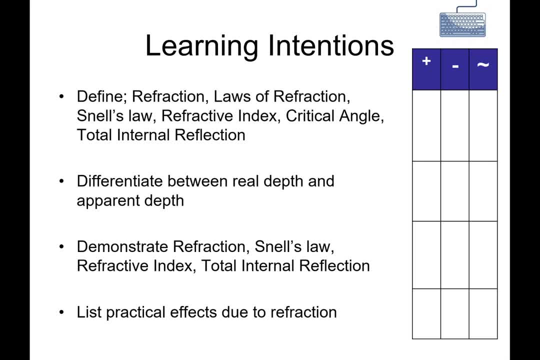 is our definitions: refraction, the two laws of refraction, Snell's law, the refractive index, what is a critical angle, and total internal reflection. So there's a few definitions that we need to go through. in this chapter. We're going to differentiate between real depth and 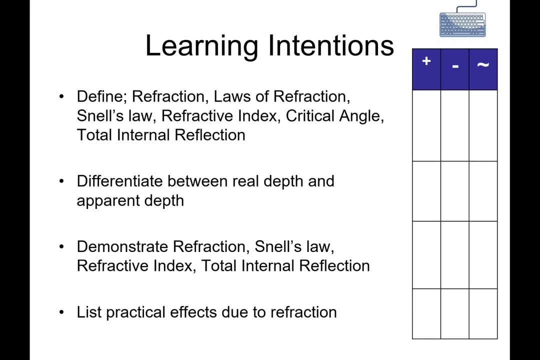 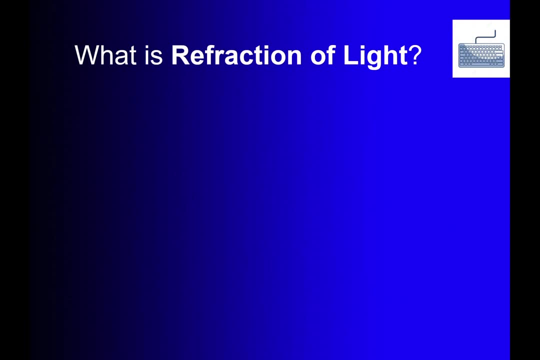 apparent depth. We're going to demonstrate refraction, Snell's law, the refractive index and total internal reflection and list some practical effects due to refraction. Okay, so what is refraction of light? I'm hoping you've seen from the first picture. there's something. 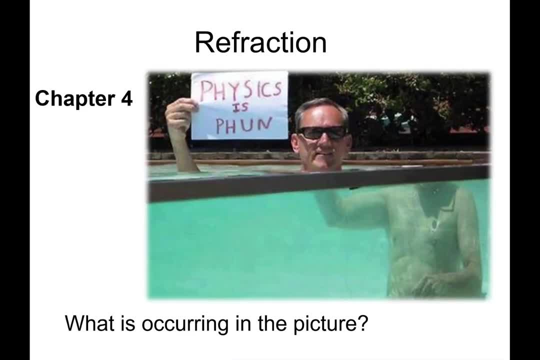 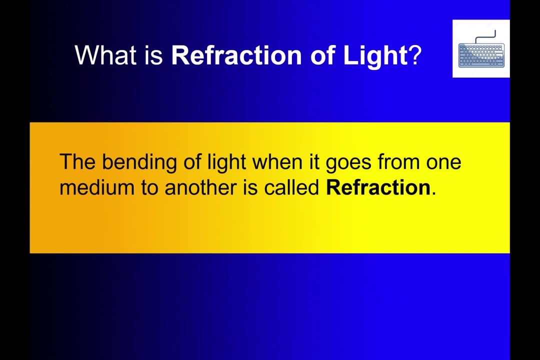 funky going on here in this picture- and we're going to have a look at what it is- Refraction is the bending of light when it goes from one medium to another. So in our first picture that we looked at there we could see light was being bent as it traveled from the water. 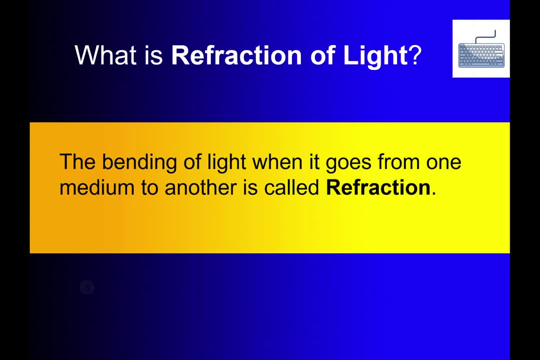 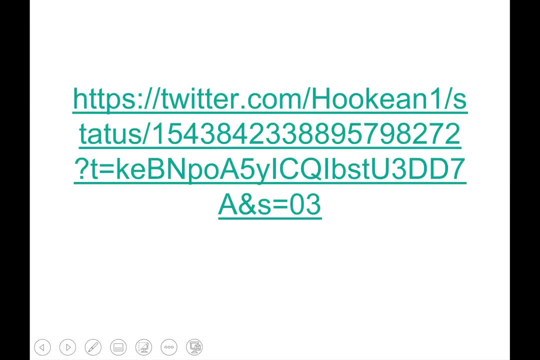 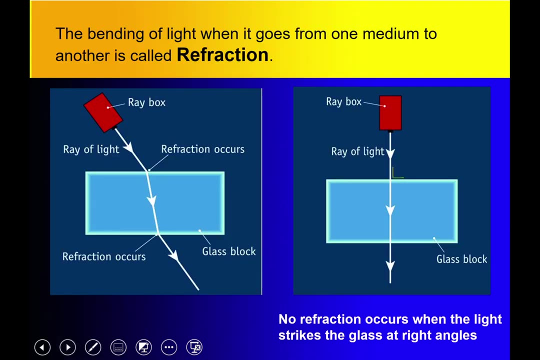 through the air to our eyes. So the light was being bent in the in some way which made it appear like this man's head was not on his body. Of course we know. we hope that's not true. Okay, so the bending of light when it goes from one medium to another is 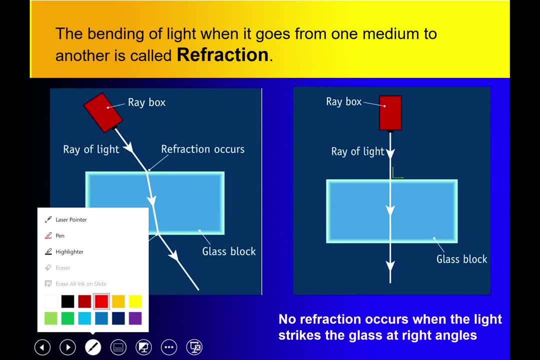 called refraction, and we can see this quite obvious in our first diagram on the left. What we've got is our setup here, where we've got a ray-box and we've got f? それ and we've got a light beam traveling from the ray box and as it hits the glass block, it starts to. 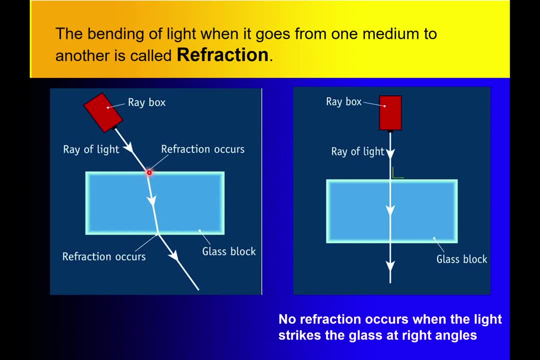 bend at this point. okay then. as it's traveling through the glass block, it travels in a straight line again, until again it travels from one medium to another. in this case it's going from glass back out to air and refraction occurs again for the second time. so we've got refraction occurring. 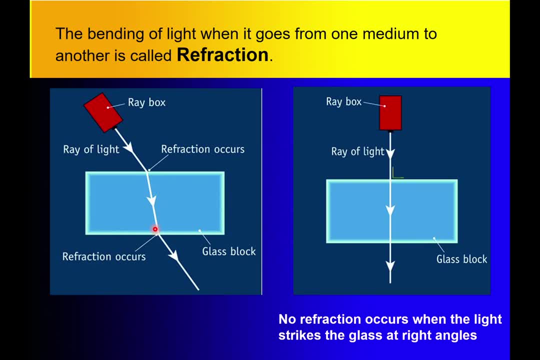 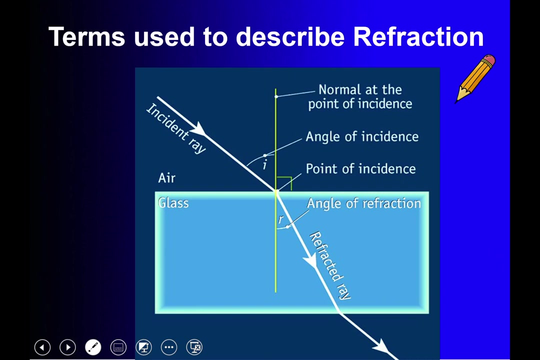 at two points here in this diagram. if we have a look at the picture on the right, we can see that the light ray does not bend in any way, or it does not refract, because the light ray is hitting the glass block at a 90 degree angle and it will not bend in this instant. okay, so some terminology that. 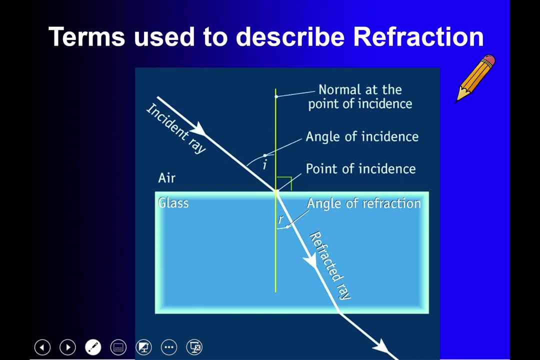 we need to be familiar with throughout this chapter. first, first up, we've got our air, where the light ray is traveling from into our glass block. second up, we've got this yellow line- excuse me, this yellow line, which is an imaginary line- that we just placed there at 90 degrees to the glass block, where the incident ray hits the glass block. so 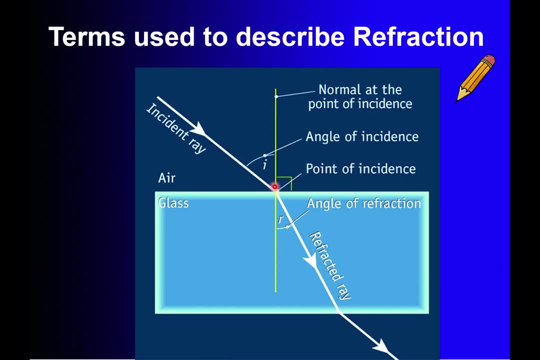 we can see at this point- we call this the point of incidence- and we've got our yellow line, which is an imaginary yellow line that we sketch, sketch at 90 degrees to the point of incidence. okay, we've got our incident ray, our incident light ray, coming in, striking the glass block at the point. 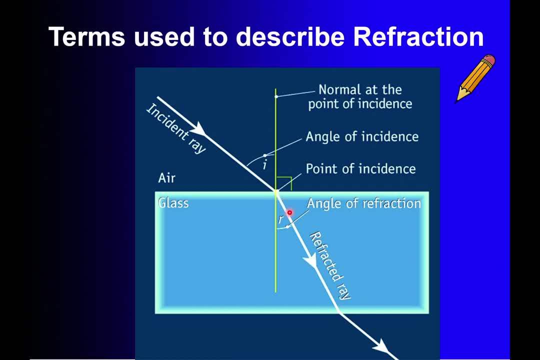 of incidence and we've got our refracted ray traveling through the glass block. okay, so the refracted ray is the light ray that has been bent as it's traveling through the glass. second and third thing to, or third or fourth thing to note is that the light ray is not bending in any way, or 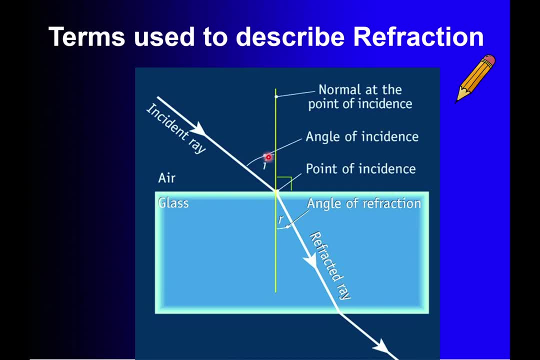 is very rather in receipt. so we're going to have to leave the ending point in the increase- hair breaking- and we're going to have to let the light ray left its position on the glass block. so now we're going to get our reality from this first tip point here and this particular self. 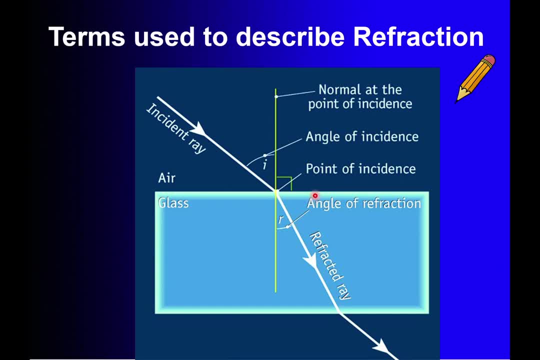 block term. and then we're going to be measuring this right angle of incidence on that angle before we go back to the glass block. and that is the angle of incidence that we're going to measure refracted ray back to the glass block. you always measure the angle towards the normal. 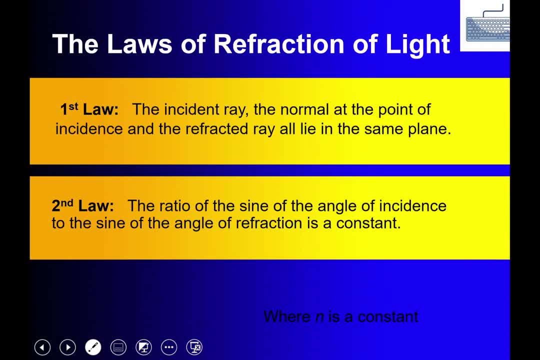 so we've got two laws of refraction, the first law being that the incident rate, the normal at the point of incidence and the refracted ray all lie on the one plane, and our second law, which is snell's law, really the ratio of the sign of the angle of incidence to the sign of the angle. 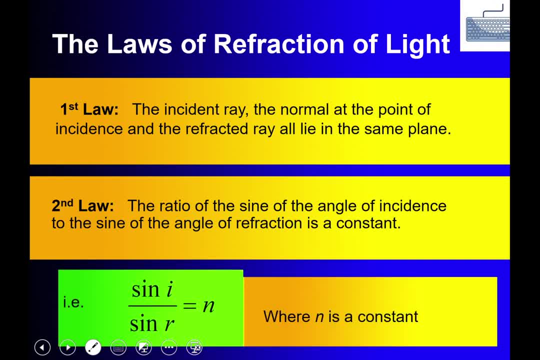 of refraction is a constant. now what does that mean? basically, the second law refers to this formula here: that the sine of the angle i over sine of the angle or it, will always give you a constant number, n, and const n is a constant, meaning that that number does not change. okay, so? 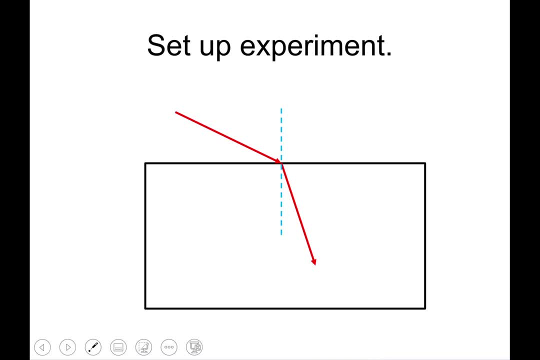 we're going to have a look at how we can verify snell's law, how we can verify that second law of refraction. what we're going to do is set up this experiment where we take a glass block and we shine a light ray into it and again we've got this dotted blue line. 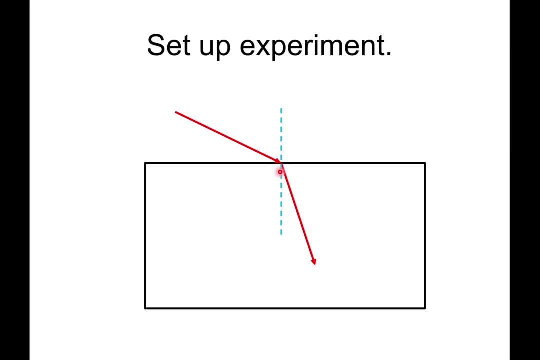 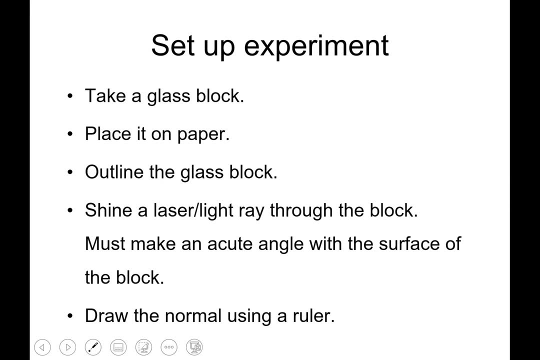 imaginary blue line, which is our normal, at 90 degrees at the point of incidence. okay, we're going to trace our glass, trace our glass block out onto the paper and we're going to shine our light ray through the block. we must make sure it's an acute angle with the surface of 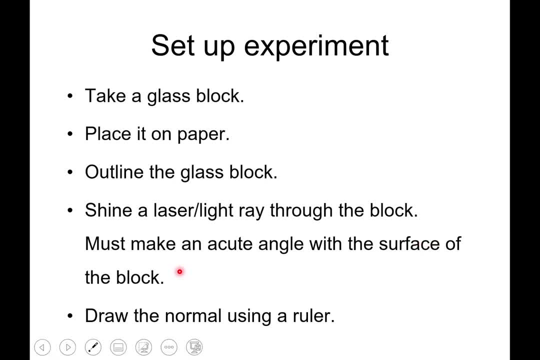 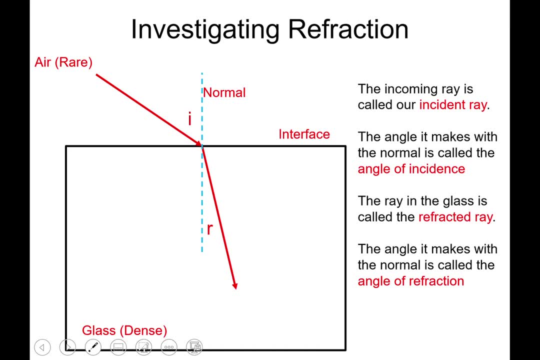 the block and we draw the normal, which is that imaginary line at 90 degrees to the point of contact and using a ruler. so this is what our investigation is going to look like so far. the incoming ray traces at our instant ray and the angle it makes with the normal is called our. 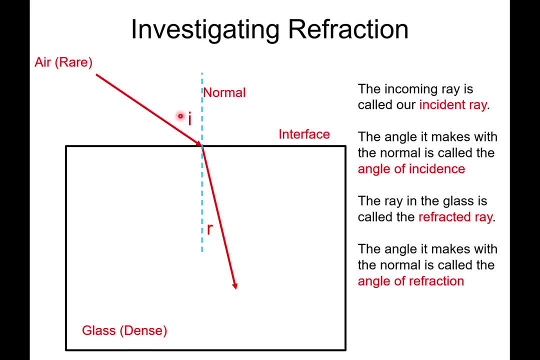 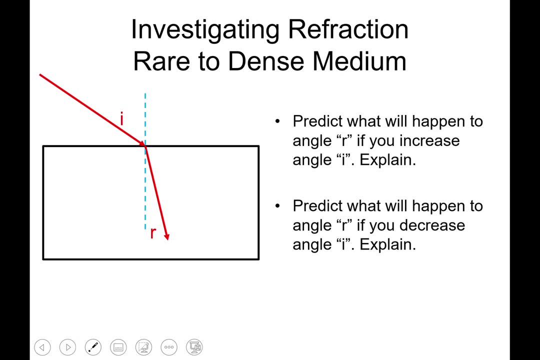 angle of incidence. that's that angle i up here, the ray in the glass is called the refracted ray and the angle that it makes to the normal is called the angle of refraction, which i'm circling right now. um, just a quick prediction. um, you guys hopefully have carried out these experiments in in class. 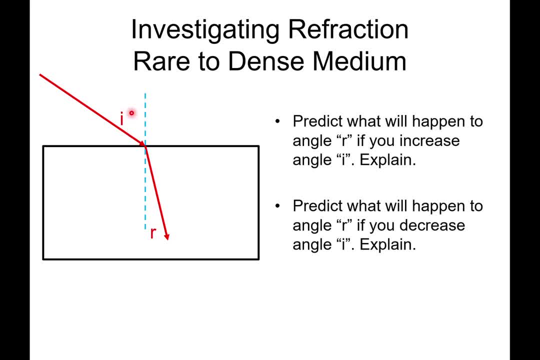 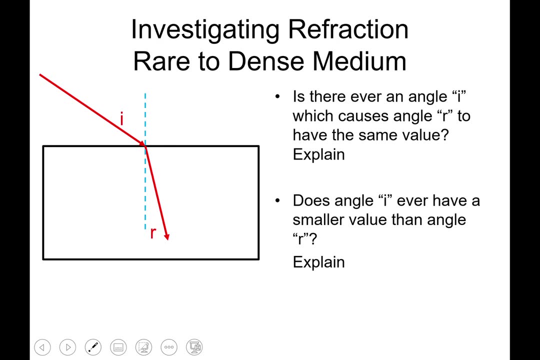 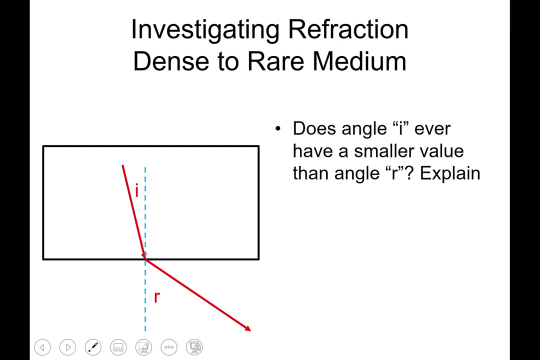 um, but i'm asking you to predict what you think will happen if angle i increases, and the answer would be that angle or increases as well. um, if angle or decreases, what will happen to angle i? it will decrease as well. Okay, we'll continue on. So when light travels from a rarer to a denser, 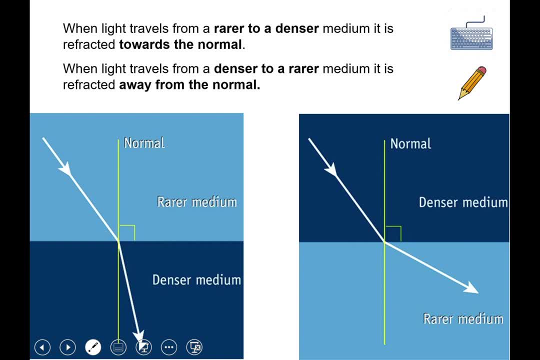 medium, it is refracted towards the normal. So let's have a look at the diagram on the left. here We've got our incident ray coming in, and if it was to travel in a straight line, it would continue the line of my pointer. However, we can see that the light ray is being bent in towards 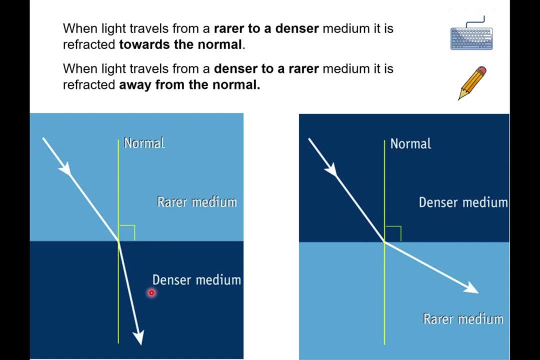 the normal. So when it's going from a less dense material to a more dense material, the light ray will bend in towards the normal. So, for example, if it's going from air to water or air to glass, it will bend in towards the normal. However, in the diagram on the right, when the light travels, 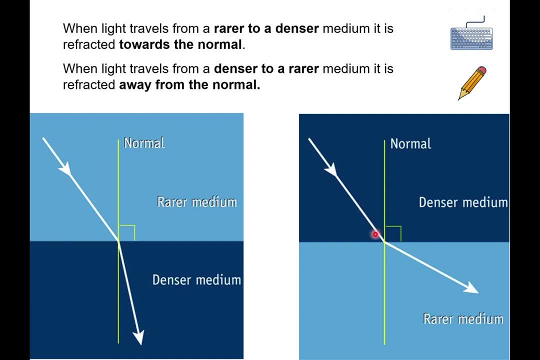 from a denser material to a less dense material, rather than continuing on on a straight path like so as if that's the line that it would take, following my laser pointer, if it was traveling in a straight line. Rather than doing that, it's bent or refracted away from the normal, So things. 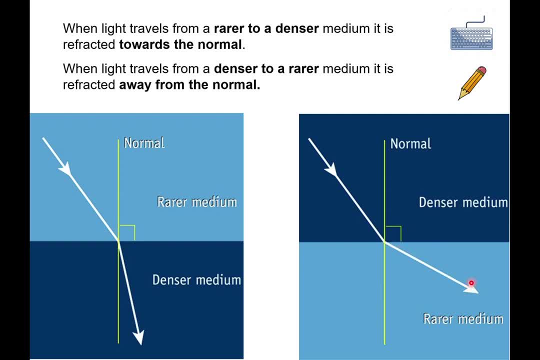 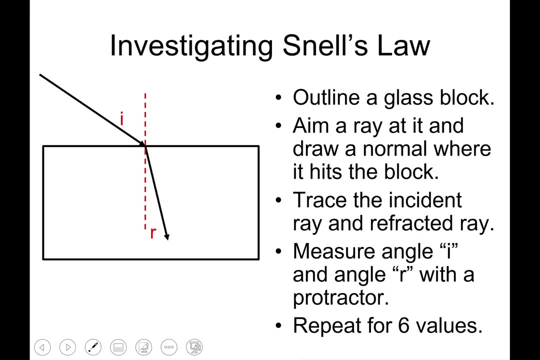 to note: when going from a more dense to a less dense, it's bent away from the normal, and when it's going from a less dense to a more dense material, it's bent. So it's going to be bent in towards, towards the normal. So how are we going to investigate Snell's Law? Well, we've outlined our glass block on. 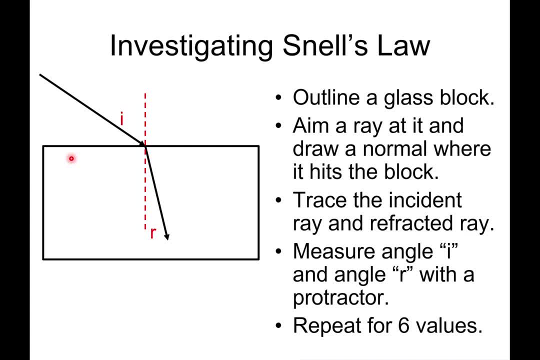 our piece of paper. We've shone our incident ray in at an angle i to the normal and we can see that it's got a refracted angle or to the normal as well. We're going to measure that incident angle i using a protractor. We're going to measure. 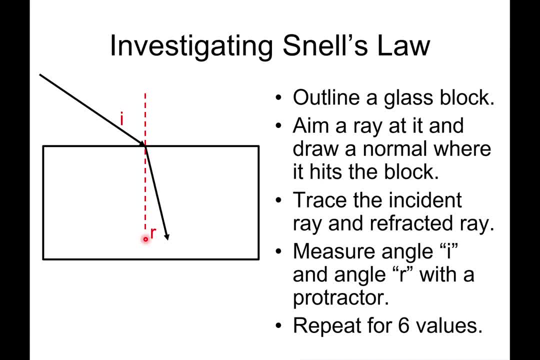 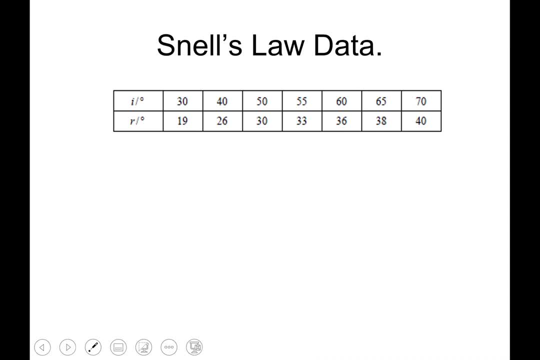 this refracted angle r using a protractor, and we're going to repeat this six times for six different values. When you do so, you're hopefully going to get a table of results that something similar to this. So if we go about plotting these results by ourselves, we see that we do not get a straight line graph. okay. 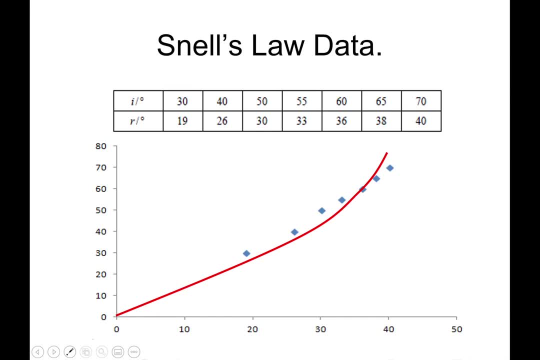 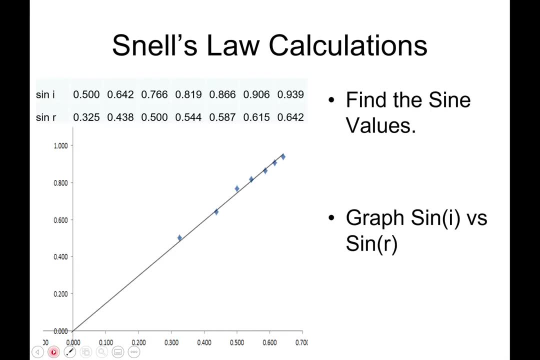 which is an issue, because if you have not got a straight line, you cannot get a slope of that line, because the slope varies at every point along the graph. However, if we get sine of our incident values and sine of our refracted values and plot sine i versus sine r, we'll 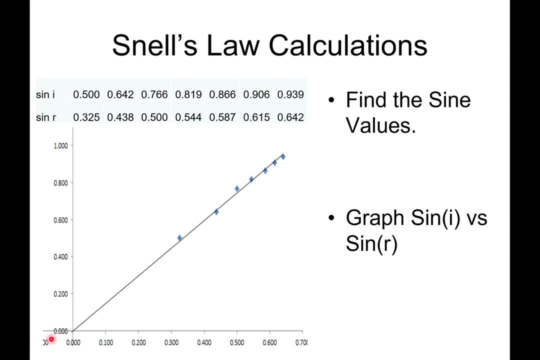 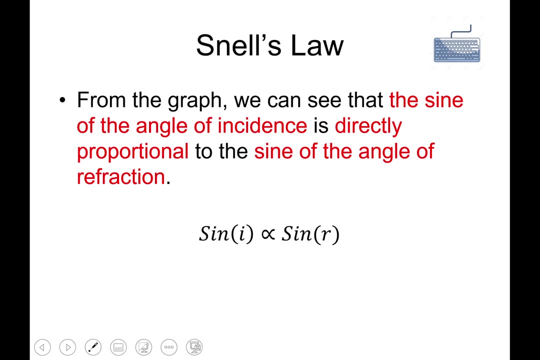 now get this location where, all of a sudden, we've got a straight line graph through the origin and we can therefore find the slope of this graph. So from the graph we can see that the sine of the angle of incidence is directly proportional to the sine of the angle of a fraction. that's what this symbol here means, that they're directly. 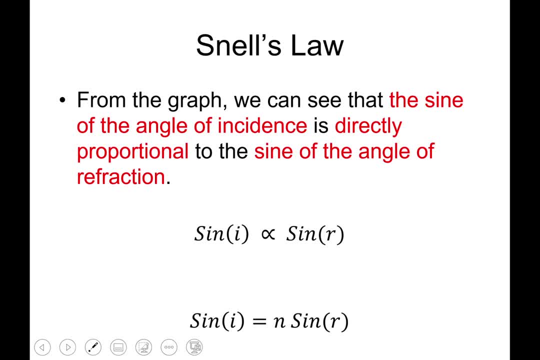 proportional to each other. Now, because just because they're proportional to each other does not mean that they're equal to each other. Why, all of a sudden, we've got a straight other. however, if we include a constant number, n, we can say that sine i is equals to sine o. 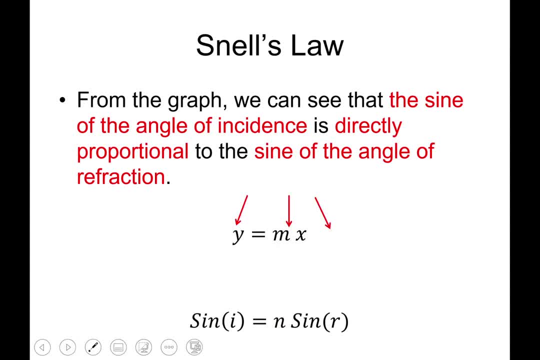 multiplied by a constant number, n. okay, so from the graph we can see that the sine of the angle of incidence is directly proportional to the sine of the angle of a fraction. so if we put sine i on our y-axis, we put sine r on our x-axis. well then, m, the slope of the graph will be equals to n. 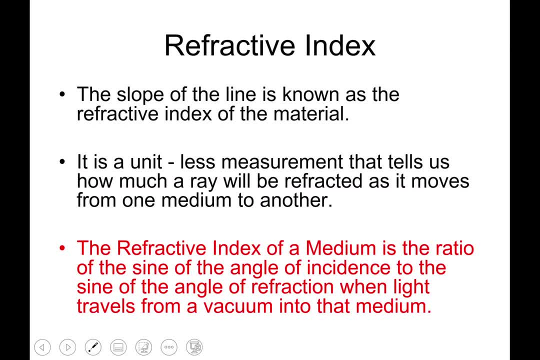 our refractive index. okay, so the slope of the line is known as the refractive index of the material. it is a unitless measurement that tells us how much a light ray will be refracted or how much it will be bent as it moves from one medium to another. 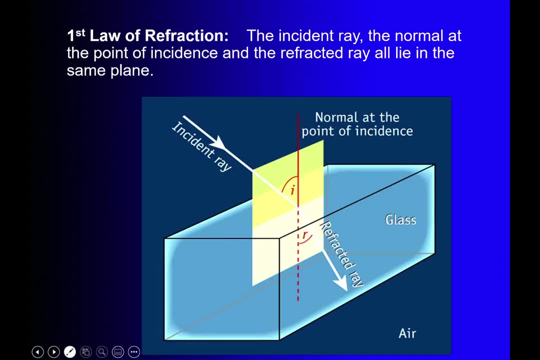 okay. so there again is our first law of refraction. we can see that our incident ray, our angle of incidence, our normal, our refracted ray and our refracted angle all lie on the one plane. so if they come in on the x-plane, they will come out on the x-plane if they were to go in on. 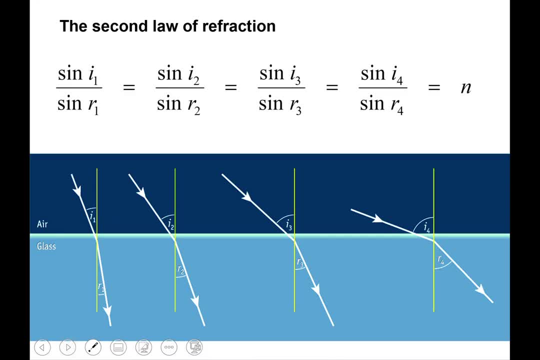 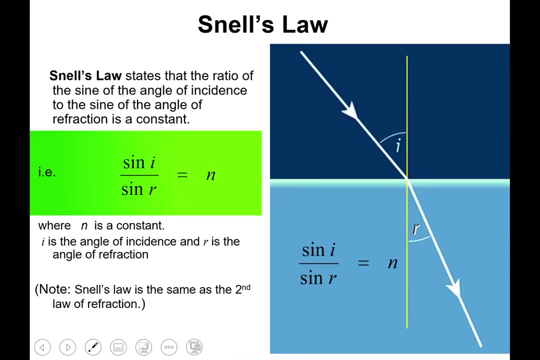 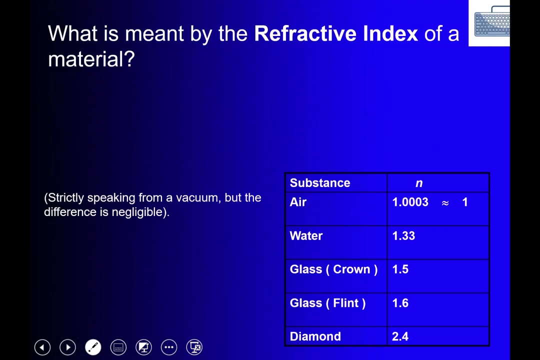 the y-plane, they would also come out on the y-plane. okay, and here's our second law of refraction. so just check what angle it is and then you will get the. okay, you can see that the refractive index over sine r is equal to a constant number n. regardless of what angle we have our incoming angle, the refracted angle will always match it to give a constant number n. okayso, 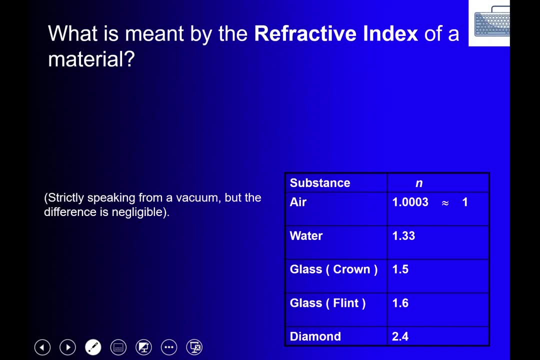 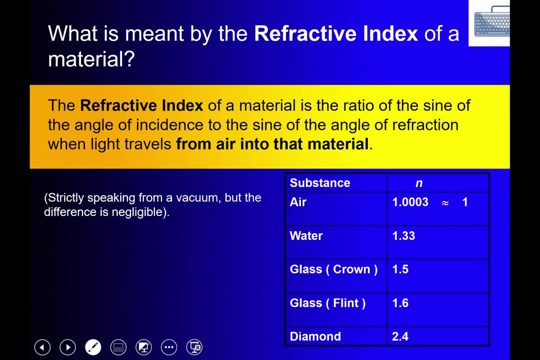 so basically the refractive index or that refractive number n is a measure of how much partnership value, crop ratio, metre or proportion ratio'll ability toн bend or can refract light. so the refractive index of the material is a ratio of the sign of the 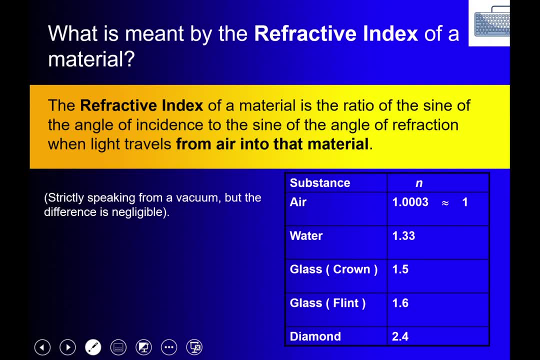 angle of incidence to the sign of the angle of refraction when light travels from air into that material. so refractive index of air is roughly one. refractive index of water is around 1.33, and of glass it varies from 1.5 to 1.6 and for diamond it's 2.4. again the refractive index. 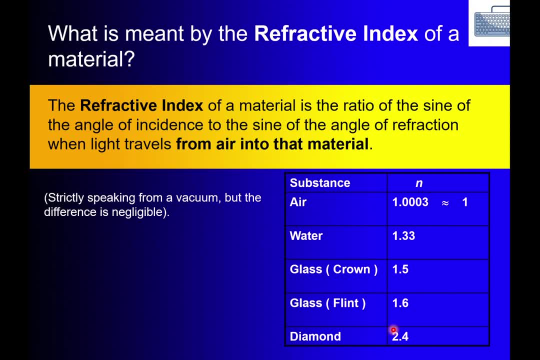 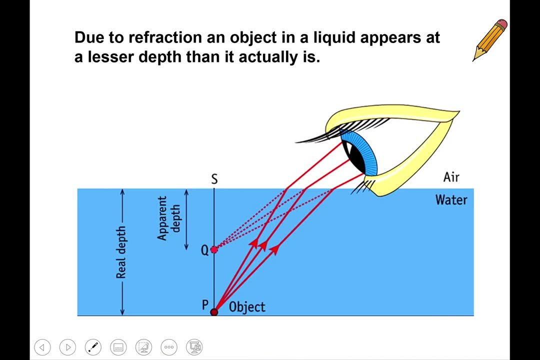 is a measure of how much that material can bend or refract the light. obviously we can see diamond can bend or can refract light the most, by comparison to water, which will bend it the least? okay, due to the refraction of an object in a liquid, it appears less deep than it actually is. 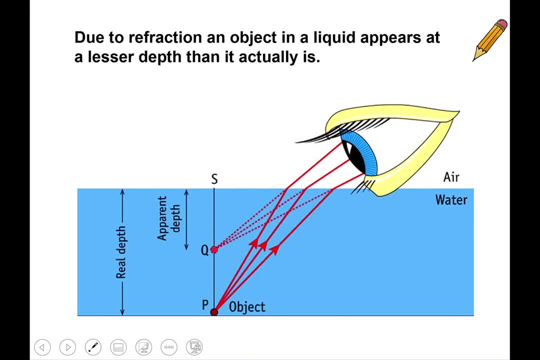 okay. so, as we now should be aware, and we can see- we've seen it in our first picture- water can bend light and, as a result of doing that, something that is underwater or submerged in water will appear less deep than it actually is when we look or when we view that object at at an angle. 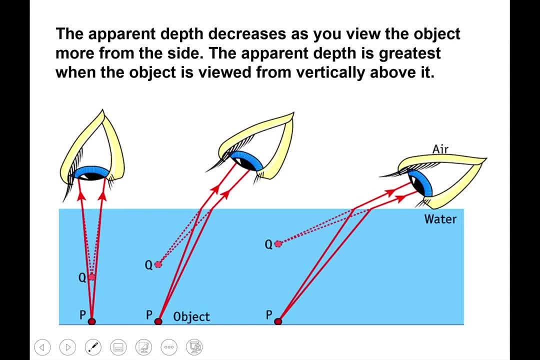 okay, so the apparent depth decreases as you view that object more from this from the side. we can see here in diagram 1 versus diagram 2 versus diagram 3, diagram 3, the object appears least deep. okay, so the greater the angle you view an object from, the more the light gets bent. therefore the more or the less deep the object. 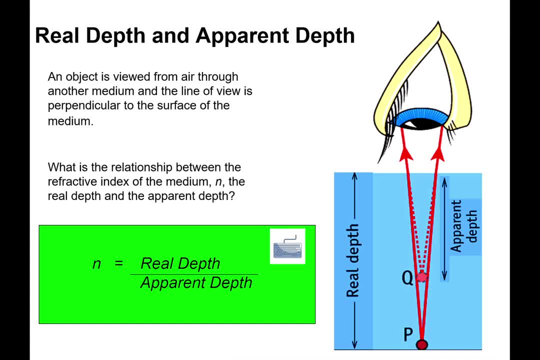 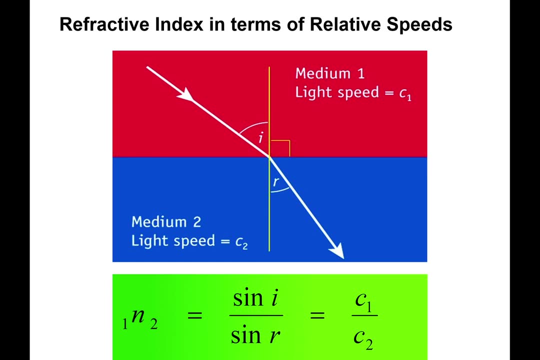 appears okay. and again we've got a formula for this. where n is your refractive index is equals to the real depth of the object over the apparent depth. okay, again, the refractive index in terms of its relative speed, light will be traveling through those objects at a certain speed. the more, the higher. 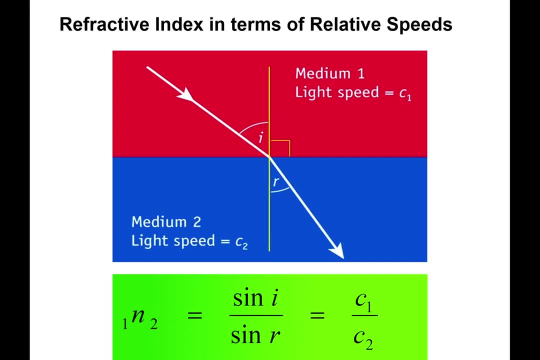 the refractive index, the greater the change in speed. okay, so you can see that the object is moving at a certain speed. so again, diamond will slow down light the most, while water will slow down light the least, but they all will change the speed at which the light is traveling through that. 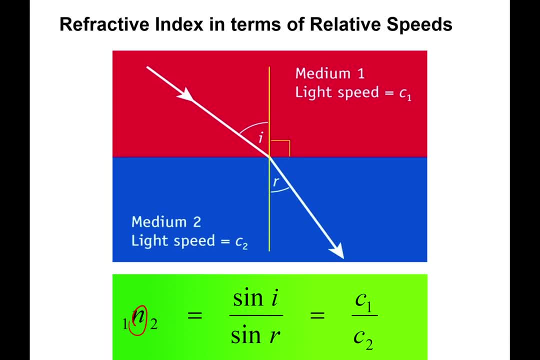 material. so again we've got our refractive index. n is equals to sine i over sine r, or it's also equals to the speed of the material in air versus the speed- sorry, the speed of light in air versus the speed of light in the material through which it's traveling. 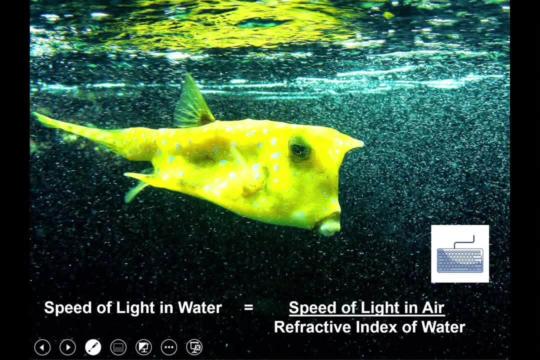 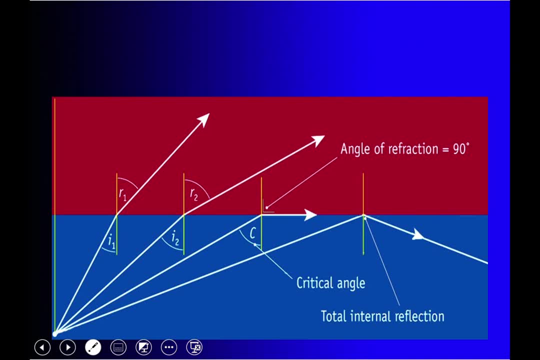 okay, and we can see. there's our formula for that. again, it's another formula that we need to be familiar with, okay. so moving on now. in this case, guys, what we've got occurring here is we've got the light traveling from a more dense to a less dense material, and we can see when it's traveling. 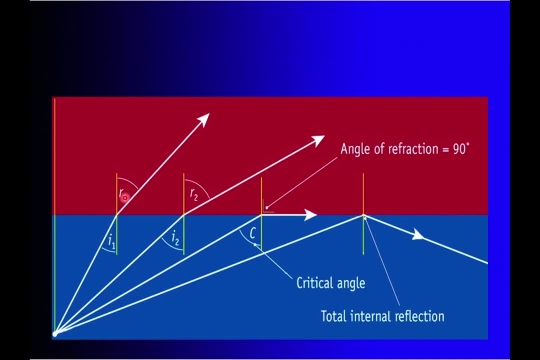 from more dense to less dense material, rather than traveling in a straight line, the light ray gets refracted away from the normal. so what's happening here is, as we continue to increase the incident angle, the light ray is refracting more and more and more. eventually you will increase. 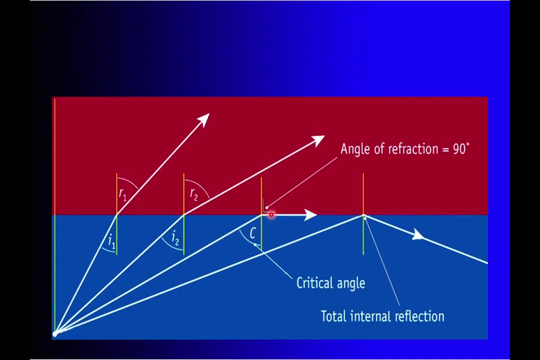 the incident angle to a point where the refracted ray no longer leaves and goes into the second material, but instead travels along the plane or along the surface between the two materials, between the water and the air. at this point, where the roof angle of refraction is 90 degrees, the 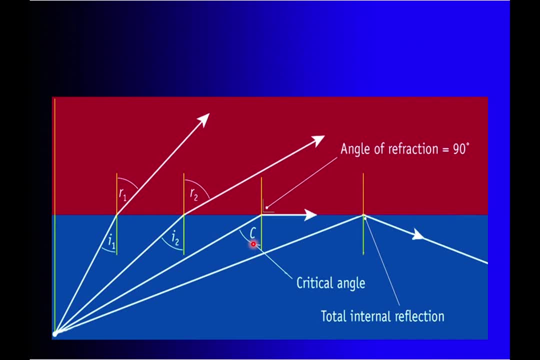 angle of incidence is referred to as the critical angle. okay, if you go beyond the critical angle, if you continue to increase your incident angle beyond the critical angle, we can see that the light ray now, rather than leaving and going into the second material, it actually reflects back into the uh, back into the material, the water. 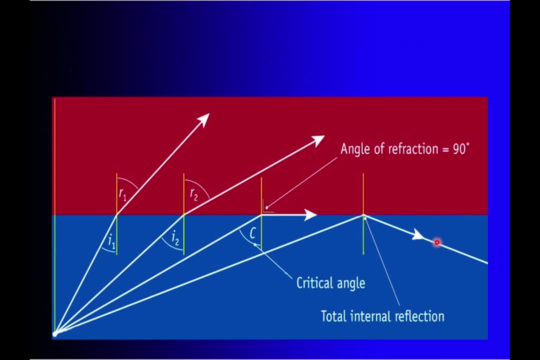 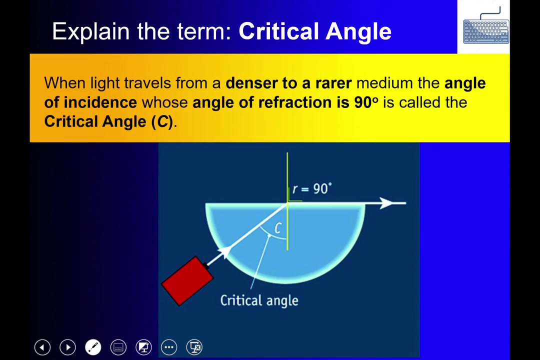 that it came, that the light ray came from. so, rather than the light ray traveling into the air, it actually reflects back underneath the water again, and this is called total internal reflection. okay, so again our critical angle: when light is traveling from a more dense to a less dense. 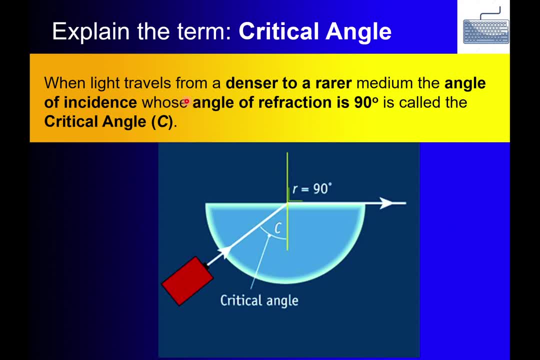 material or medium. the angle of incidence whose angle of refraction is 90 degrees, is called a critical angle. so when we change the angle of incidence to an angle of time, we can see that the light ray is showing a critical angle when light is traveling from a more dense to a less dense material. 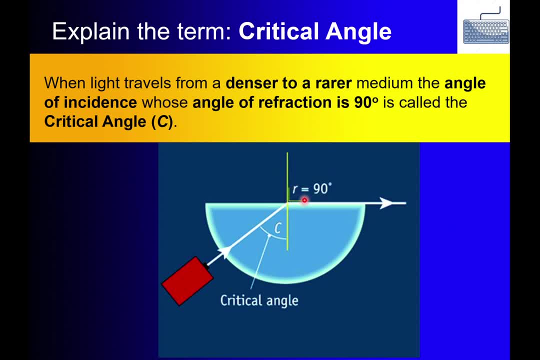 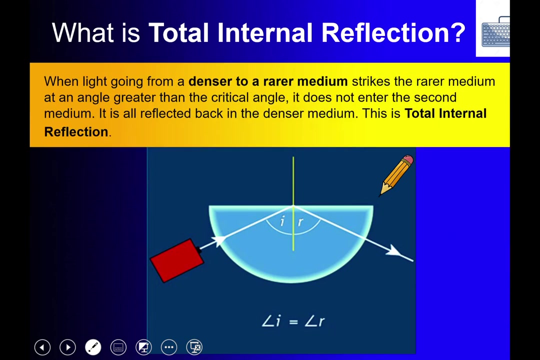 we can see here, our angle of refraction is at 90 degrees to our normal, and therefore the corresponding angle of incidence is referred to as the critical angle. so the critical angle is the angle where the refracted angle is equal to 90 degrees when light is going from a more dense 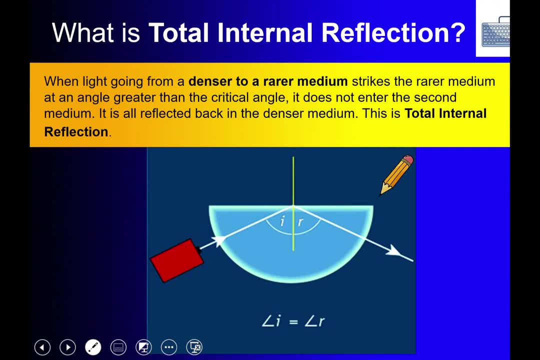 to a less dense material and it strikes the rarer medium at an angle greater than the critical angle. it does not enter the second medium or the second material. instead, it's reflected back into the denser material and this is known as total and terminal reflection. so we can see we've gone beyond the critical angle here now and our light is now rather than 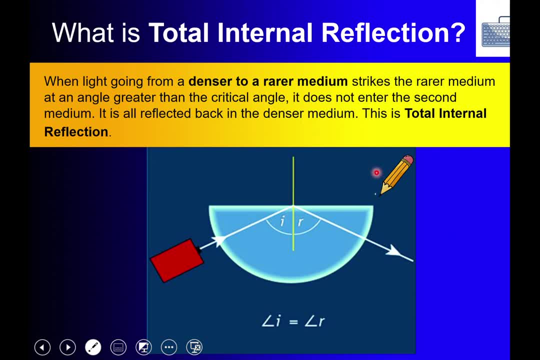 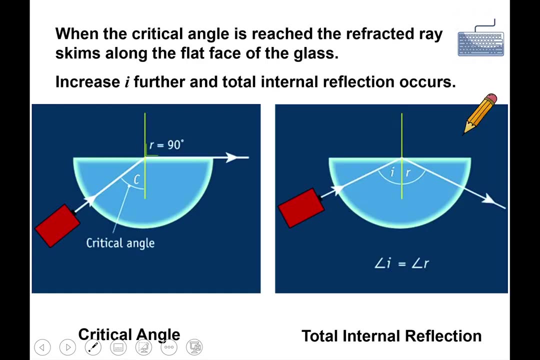 heading out into our second medium, into the air. the light ray has been reflected back into the glass again, and this is known as total internal reflection. okay, so hopefully in class again, you would have set up this experiment where we seen whereby light um is shone through a semicircular glass block and what's happening is we've reached a critical 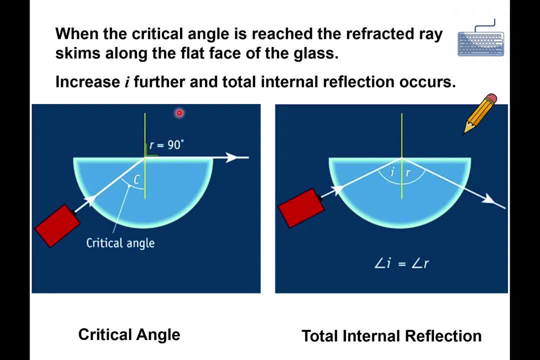 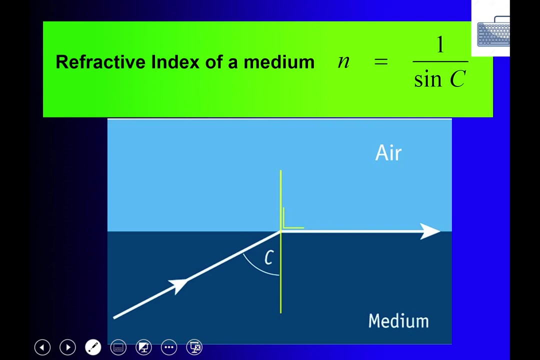 angle here now where, instead of the light traveling out into the air, it's just traveling along the surface of the glass block. if you continue to increase that critical angle, what's instead happening is total internal reflection is occurring, the light rays traveling back into the glass block. so we've got another formula for this again, where n the refractive. 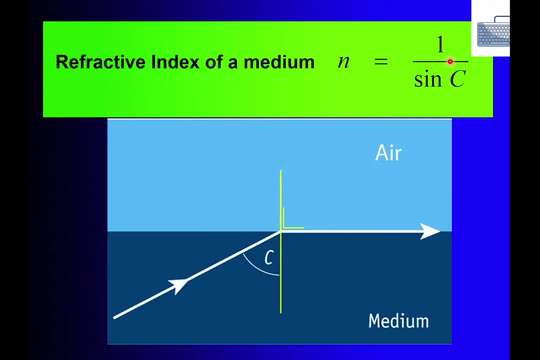 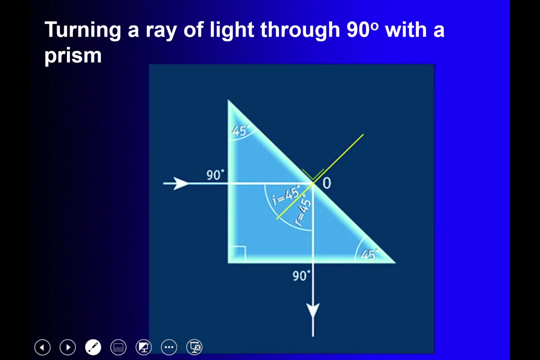 index of that material is equals to one over the sign of our critical angle c. so if you know the critical angle c, we can find the refractive index, or vice versa, if you know the refractive index, you can find the critical angle of that material. now we can use this phenomenon to bend light through 90 degrees using a glass prism. 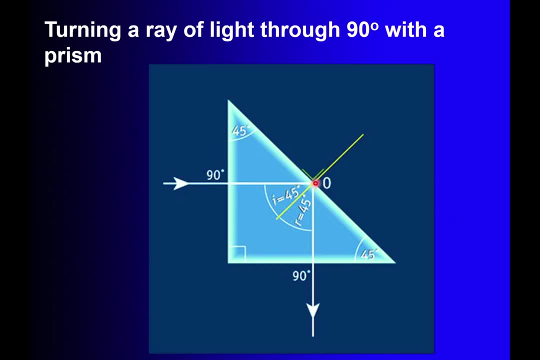 so what we've got here is a light ray coming in, striking on the surface of our prism at an incident angle of 45 degrees and, rather than it passing back out into the air, it bends back into the glass, uh, reflects back into glass at an angle of 45 degrees. 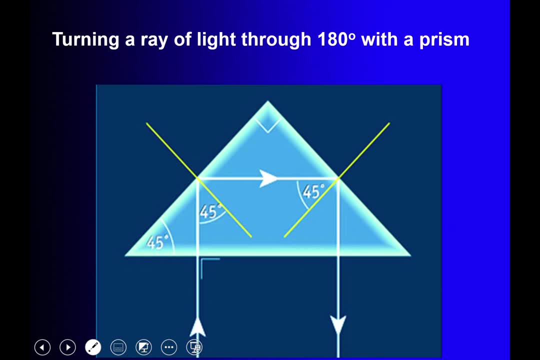 we can also use this to turn a light ray at 180 degrees. so we've got a light ray incoming here again strikes our angle of 45 degrees rather than heading back out into the air. so we've got a light ray that totally internally reflects, hits this other surface of the glass. 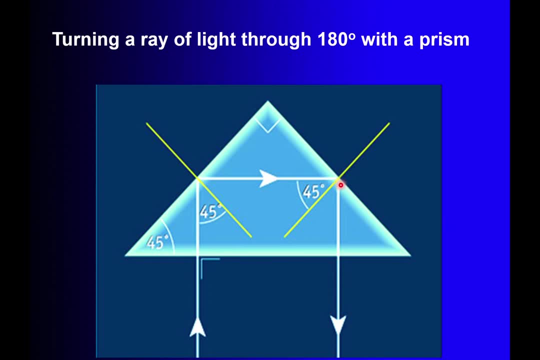 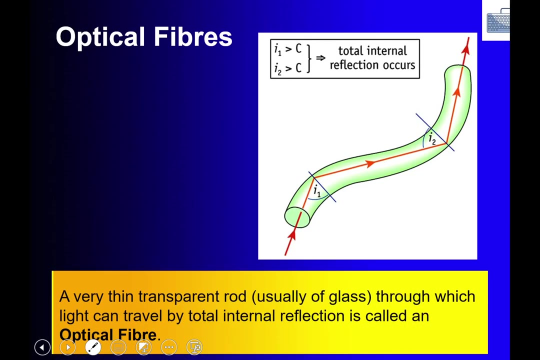 again. rather than leaving and heading back out into the air, it bends again or reflects again at 45 degrees and travels back out. and here we've turned our light ray by a total of 180 degrees. okay, using this phenomenon, we have created things like optical fibers, which are very thin, transparent. 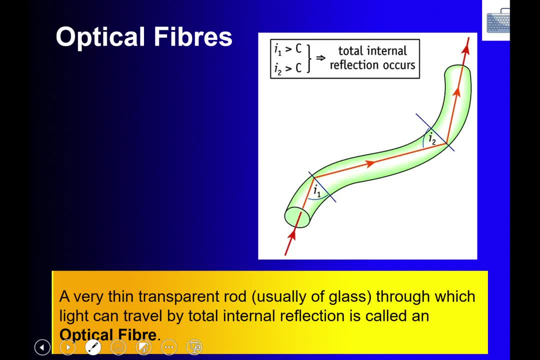 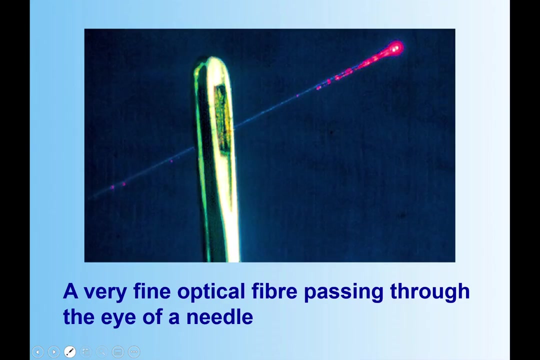 usually made from glass, through which light can travel by total internal reflection. so fiber optic cables: how our broadband, hopefully, is coming into the majority of our homes is through our fiber cables and that is these transparent rods which um light can totally internally reflect through. so here's an idea of how small these fiber optic cables can be where we've got light traveling. 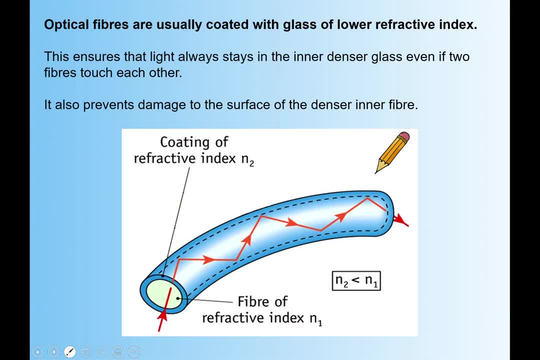 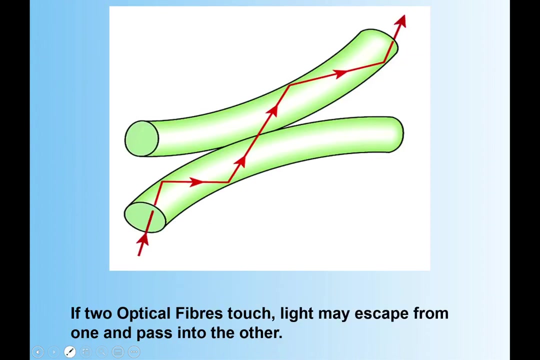 through the eye of a needle. okay, so the key thing to note with these fiber optic cables, guys, is that they are not hollow cables, they are- um, they are hole. they are made from glass, which allows light to just travel. true, and we can see here what we've got, rather than just, uh, if we hit two fiber optic. cables touching the light hasn't berabered through but kind of stopped karena that's probably the final algorithm we chose here, because, as you see here with the fiber optic cables guys have some sort of we can get this going through the eye of a needle, okay. so the key thing to note with these fiber optic cables: 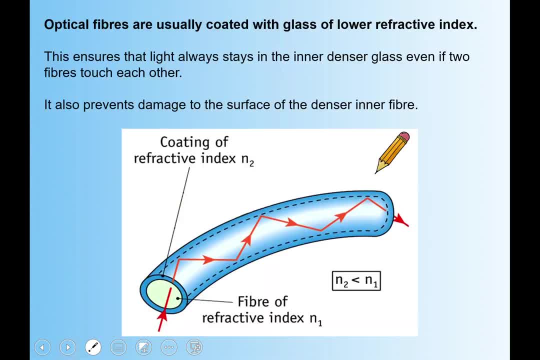 light may escape and pass from one to another. so what we do to ensure this doesn't happen is we put a coating around these fiber optic cables and this ensures that the light travels or continues to bounce or totally internally reflect through uh the cable and it also. 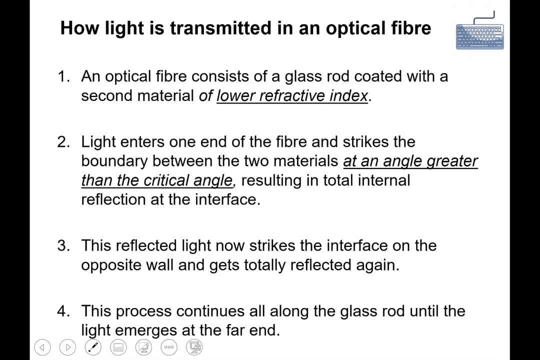 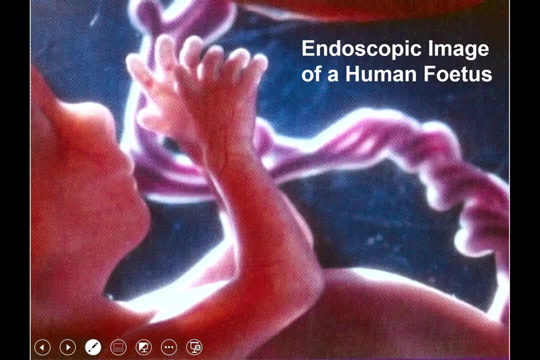 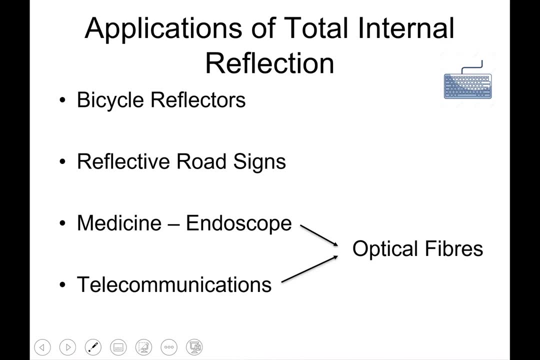 prevents damage to the inner, the inner fiber. okay, so some uses of this are endoscopic images of our fetuses or of a fetus and we can be used through in bicycle reflectors and reflective road signs and in telecommunications, as we mentioned already. so these are all applications of total internal reflection. okay. 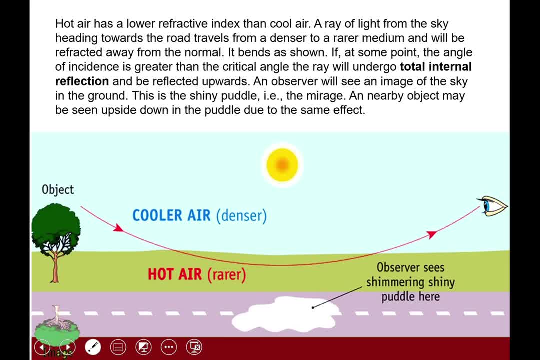 a mirage is also another example of how total internal reflection can occur, whereby when you see a shiny puddle or what looks like a shimmer on the um on the ground, that's actually what you're seeing. is the sky above you. okay, so images are being totally internally reflected back onto. 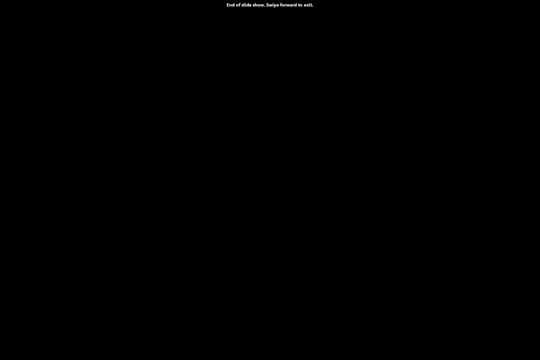 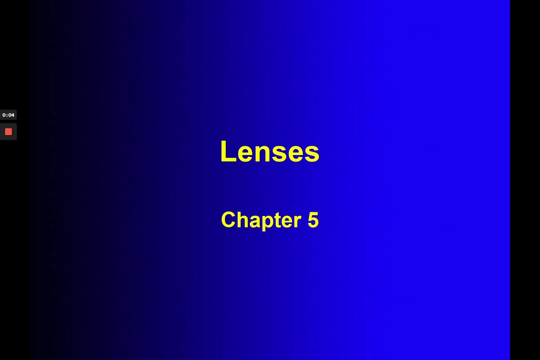 the ground. so, guys, i hope this helps you with a better, or gives you a better, understanding of refraction, um, and thank you very much for watching. okay, guys, welcome back to the second half of this video. we're continuing on from refraction and we're going to have a look at lenses now. so our learning intention is: we've got a couple of 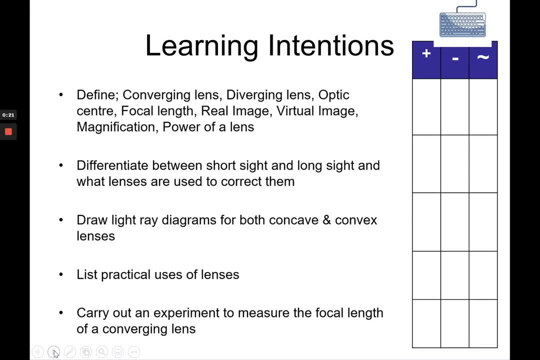 definitions- again quite a few definitions in this video that you guys need to become familiar with. firstly, what a converging versus a diverging lens is. the optic center, the focal length, real image and virtual images- we would have touched on them in previous chapters. magnification and the power of a lens. you need to be able to differentiate between short-sighted 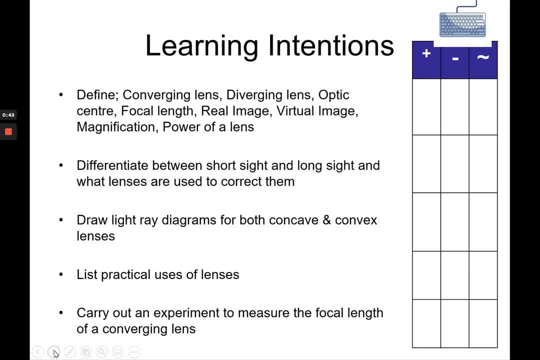 and long-sighted, and what lenses are used to correct both of these defects, and we're going to draw light ray diagrams for both concave and convex lens, practical uses for lenses- and you've got an experiment to measure the refraction and the conceptuality of that and i'm going to show you. 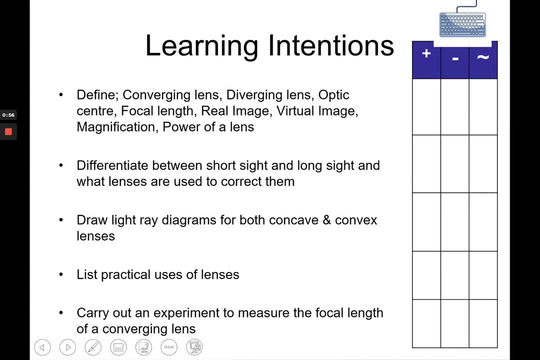 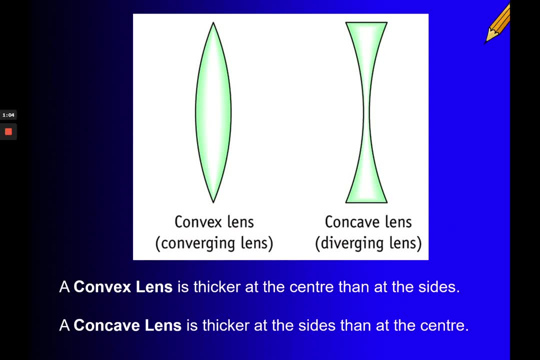 measure the focal length of a converging lens. so up next, we've got a difference here between the two: what's a converging lens versus what's a diverging lens? okay, we can see. firstly, on the left, here let me get my pointer. here we've got our converging lens, also known as a convex lens. 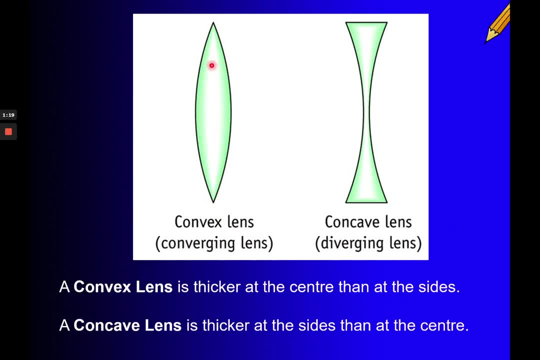 it's thicker at the center and narrower at the top and the bottom, versus our concave or our diverging lens on the right. here it's thicker at the top and the bottom and it's um caving in at the center. okay, also known as a diverging lens. 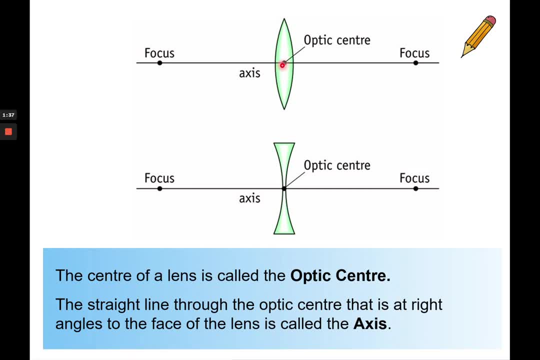 so the optic center in both cases, guys, is the very middle point of the lens. again, we've got our principal axis traveling straight through our two lens and our optic optic center is that center point where the uh principal axis travels through the center of the lens. um, again, rather than just having one focus, we've got a focus either side of our lenses. 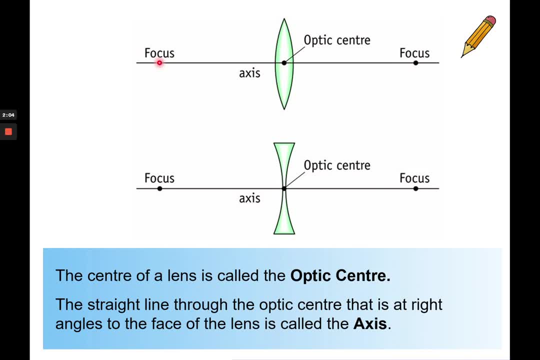 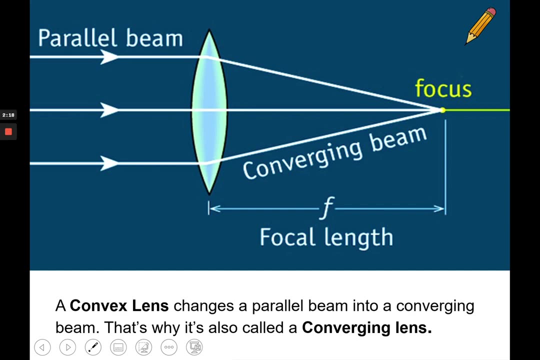 now, guys, and be aware, the distance from the focus to the optic center. if it's 10 centimeters on one side, must also be 10 centimeters on the other side. they're the same distances. make sure when drawing these diagrams you measure that out correctly. so a convex lens, or it's known as a, 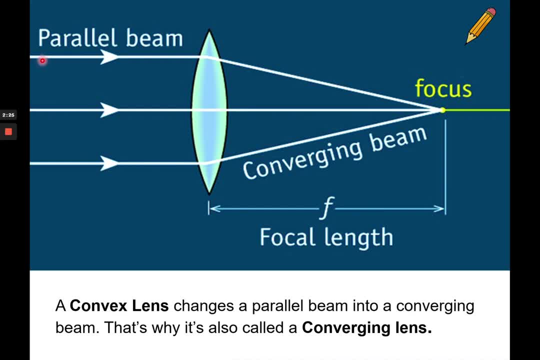 converging lens. the reason being: we can see here, we've got parallel light rays traveling in and what happens is these light rays converge at a single point. they're converging at the focal point, okay, hence why a convex lens is also known as a converging lens. 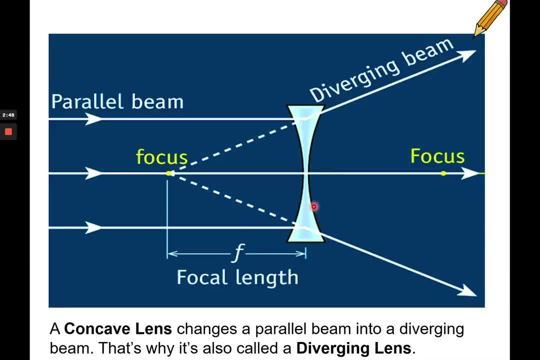 up. next, we've got our concave lens- easy to remember because it caves in at the center- as a diverging lens, because while we've got three light rays traveling in here, rather than the three of them converging out of the focus like they did earlier on the, in this case they're diverging light. 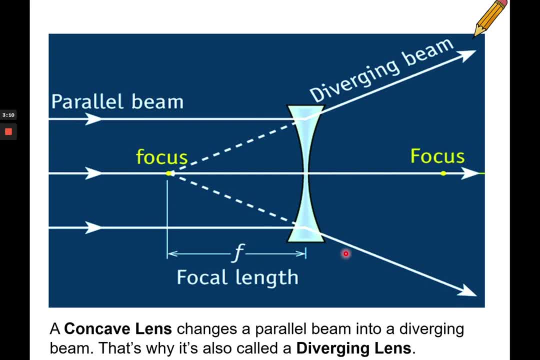 the diverging, the three light rays. now, if you were to trace these light rays back, backwards, like we've done in previous chapters, you'll find that they converge behind at the focus again, or at that, our difference between our converging on, our diverging lens. okay, now, like with our mirrors. 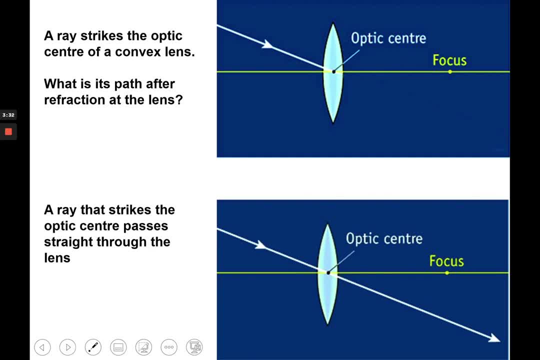 we've got some rules or some laws that we need to follow. i need to be aware of first up. if we've got a light ray coming in and it strikes the optic center, it travels straight on through. it does not bend or does not um. it does not bend or refract in any way. however, if we've got a light ray, 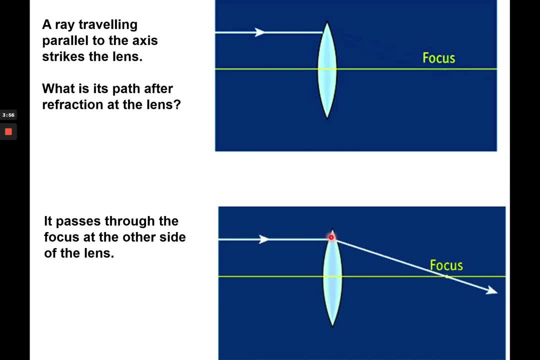 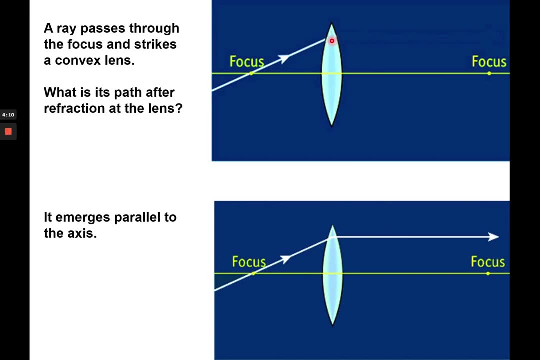 traveling in parallel to the principal axis. when it travels through our converging lens, parallel to the principal axis, out through the focus on the far side. okay in this case, if we've got a light ray coming through the focus and then hits our converging lens, if it comes through the 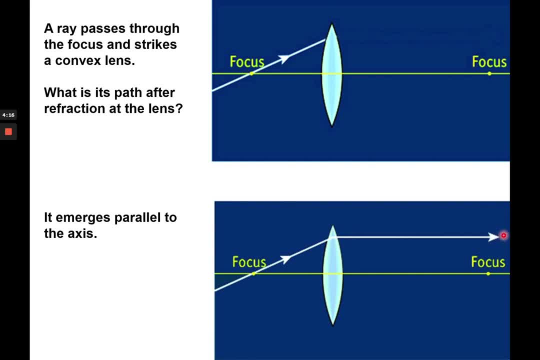 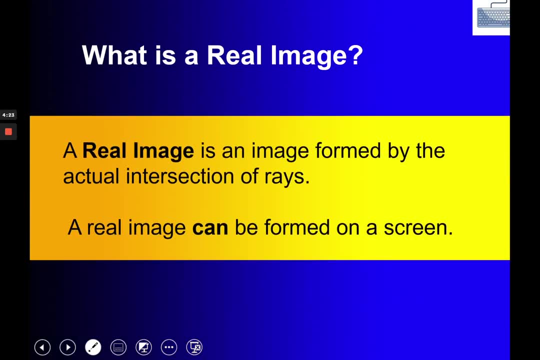 focus, it comes out parallel to the axis on the other side of the lens. so again, a real image, guys, is formed by the actual intersection, and that word actual is very, very important. um, that is a real image. okay, a real image, like with our mirrors, can be projected onto a screen. 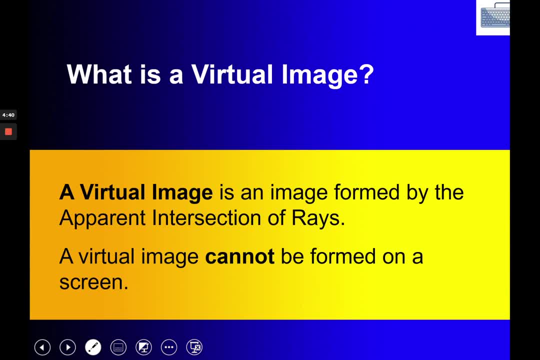 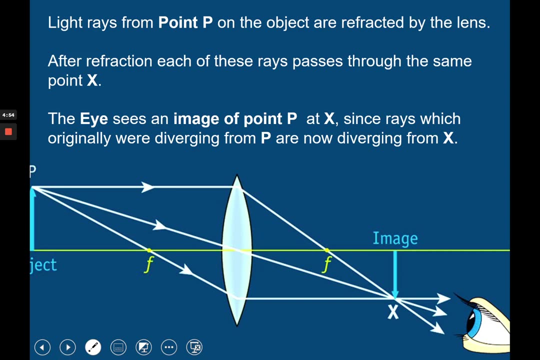 a virtual image is formed by the apparent intersection of light rays, and that word apparent is the key thing here, guys. it's the apparent intersection of light rays that cannot be projected onto a screen, so leave that for yourself. the Джomex: it occurs when an object is being looked at from one side of the lens. 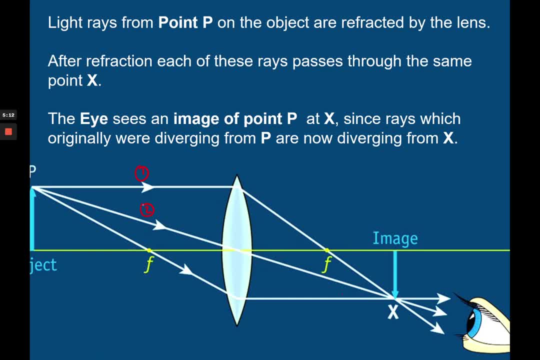 okay. so what we're going to have a look at now is a couple of diagrams showing how we've got an object on one side of a lens and where the image is going to form. okay, so we've got three light rays here. all right, just label them. 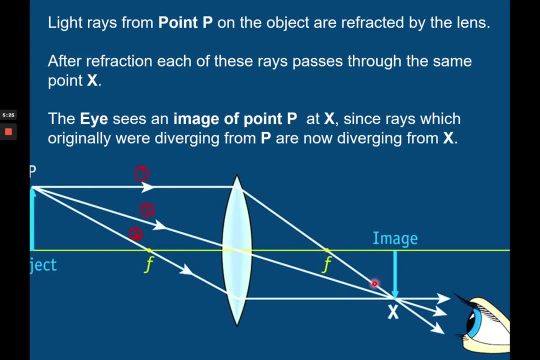 so comes out through the focal point on the far side of the lens. light ray through. light ray 2 travels straight straight through the optic center, does not diverge or does not bend in any way, travels straight on through and light ray 3 travels through the focal length and, if it, 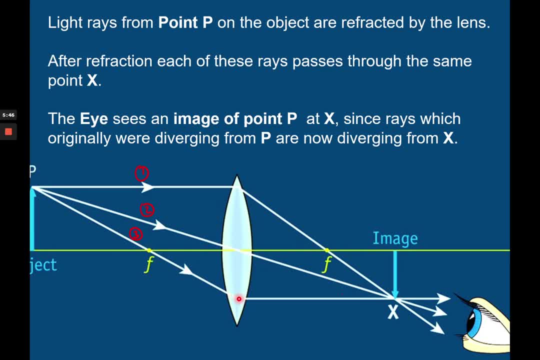 travels through the focal length or focal point, hits our hits, our lens, travels out parallel the same parallel to the principal axis on the other side of the lens. now, where our light rays intersect, is where our image is going to form and we can see a position x. here is where our light 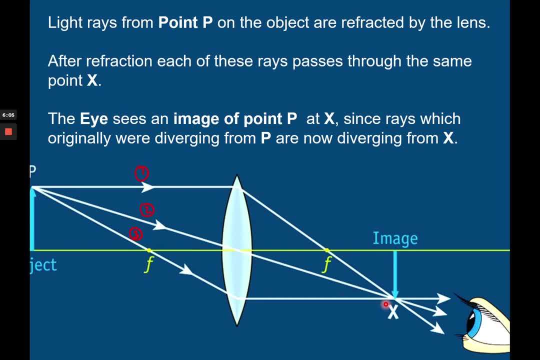 ray. our light rays intersect, so there is where our image is going to form now, similar to our mirrors. we notice in this case the image is below the principal axis, while the object is above the principal axis, our image has been inverted or flipped upside down. what we'll also notice is our image is. 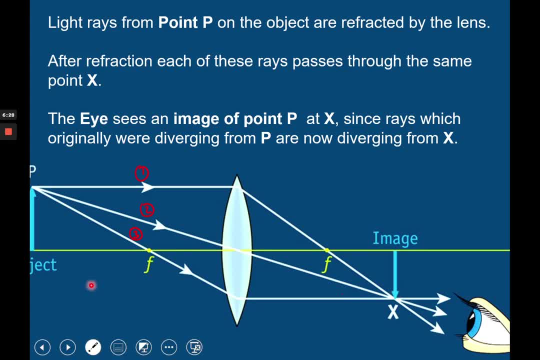 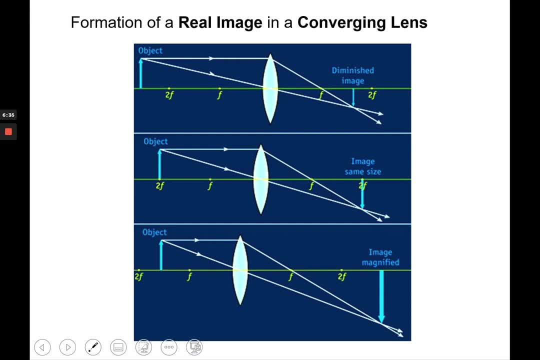 slightly smaller, so it's been made a little bit smaller as well. okay, up next, guys, like with our mirrors again, depending on where our object is positioned, and just get a pen. we've got diagram one, diagram two and diagram three. we can see, depending on where our object is positioned, our image will form slightly differently. so in diagram one our 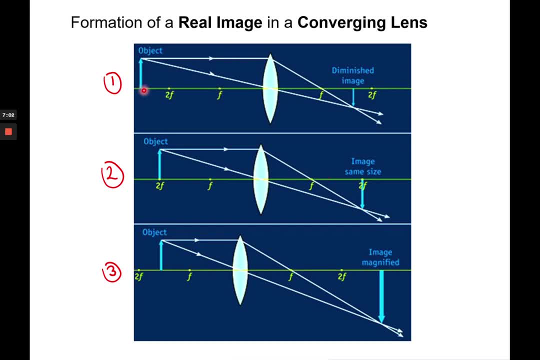 object is behind two times the focal length and our rules never change. in parallel to principal axis uh, through the focal point, through the optic center, does not, does not change its course, and we can see that here our image is diminished. if our object, however, is placed on two times the 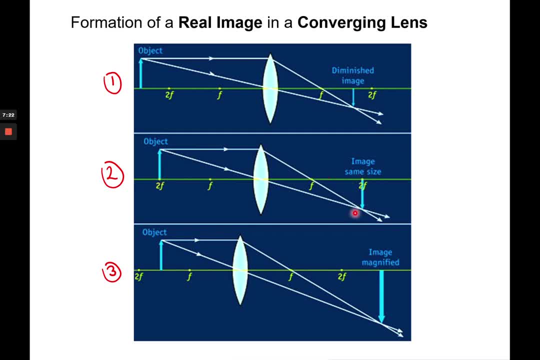 focal length. it still is inverted, it's still upside down, but it comes out at position two times the focal length on the far side of the lens, the same size. however, if the object is placed inside two times the focal length, well then, remember our light rays. our rules never change. 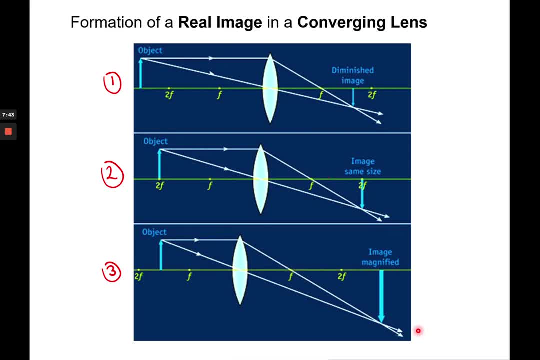 in parallel to the principal axis, out through the focal point on the far side, through the optic center, does not diverge, does not bend in any way, does not bend in any way, does not bend in any way, straight through where our light rays intersect, is where our image is going to form, and in diagram, 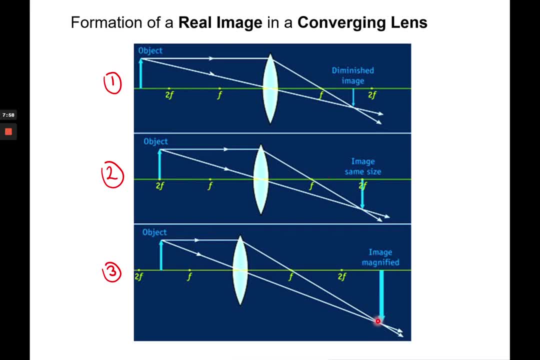 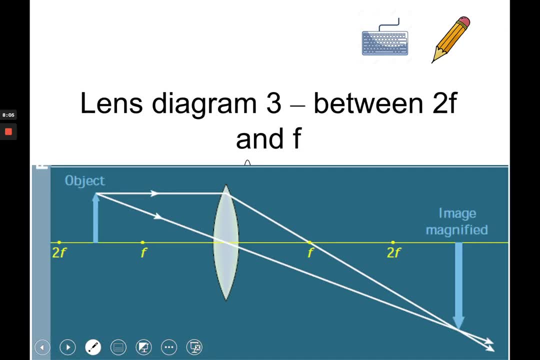 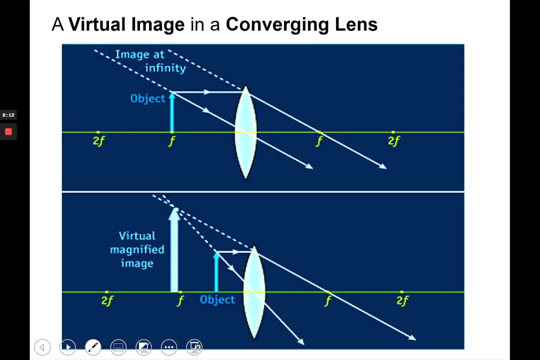 three down the bottom we can see. in this case our image is magnified, so that's just detailed view at those three diagrams. guys, you need to be aware we need to be able to draw these diagrams, so practice doing that now. again, if we place our object, 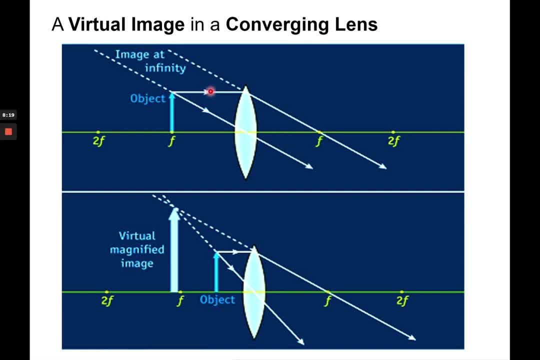 on the focal length. something funny happens: your rules never change in parallel, out through the focal point, through the optic center, does not diverge and what you see here is we've got two parallel lines. parallel lines, they never intersect, neither going forwards nor going backwards. so therefore that will always be an image at infinity, meaning the image will be blurry. you'll never get. 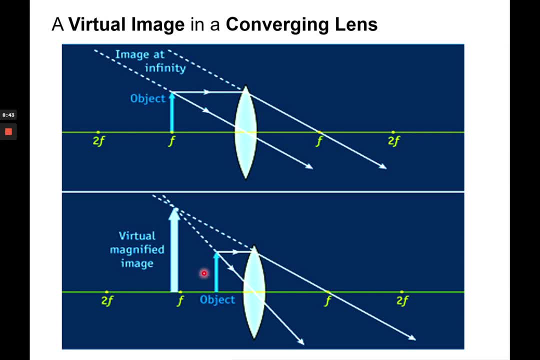 a clear image forming. however, if you take your object inside the focal length, like we can see in our second diagram here, something else happens. rules never change. in parallel to the principal axis, out through the focal point, through the optic center, continue on the same path does not diverge in any way. on the far side of our lens we can see these light rays. 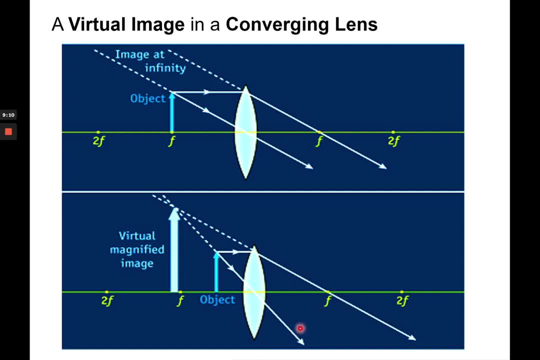 are diverging. they're getting further away from each other, so they're not going to meet behind the lens. on the right hand side of the lens, however, if we trace these backwards, we can see that the will eventually intersect now, because it's the apparent intersection due to these dotted lines here. this is a virtual image and it's going to be magnified. 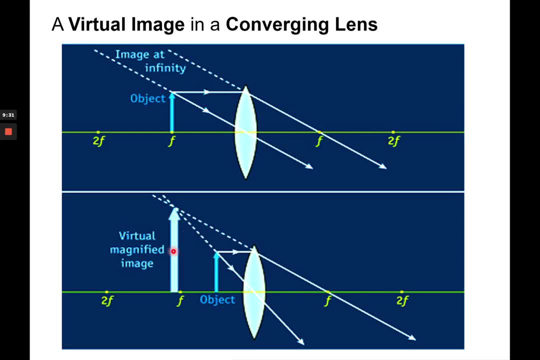 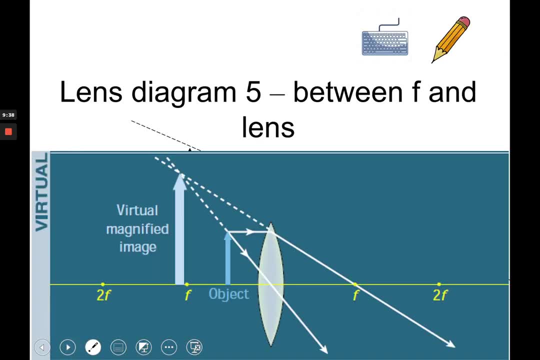 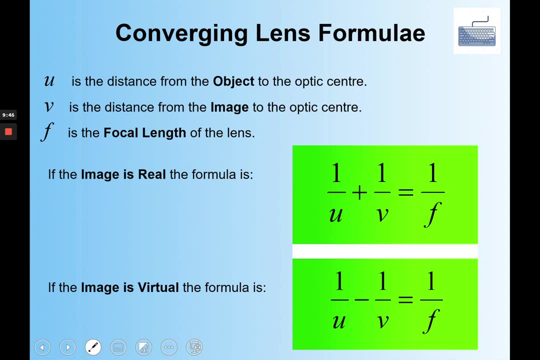 we can see. it's upright, it's magnified, but it's a virtual image. this cannot be projected onto a screen again. that's those two diagrams, again in detail. need to be able to draw these diagrams, guys. okay, so our formula now for our converging lens. nice and simple. this, well, it's in. 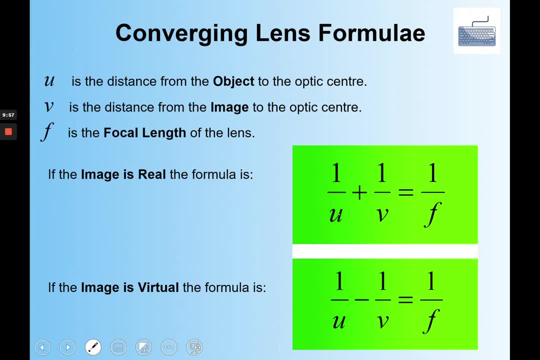 our log tables, so that will help us out. certainly. 1 over u plus 1 over v is equals to 1 over f. f represents the focal length, u represents the distance from the object to the optic center of the lens and v represents the distance from the image. 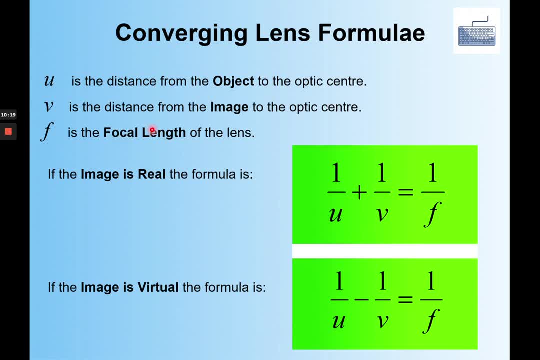 the optic center. okay so, and then f is the distance from the focal point to the optic center. if it's a real image, we've got a positive in front of our image v. if it's a virtual image, it's going to be a negative in front of our image v. 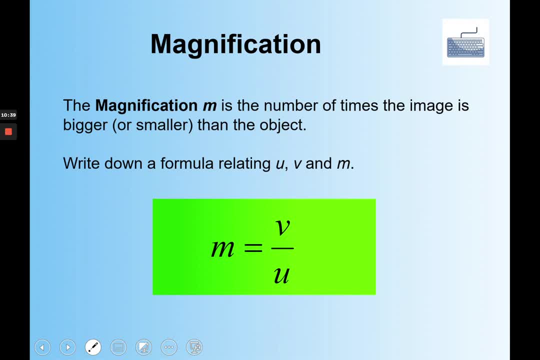 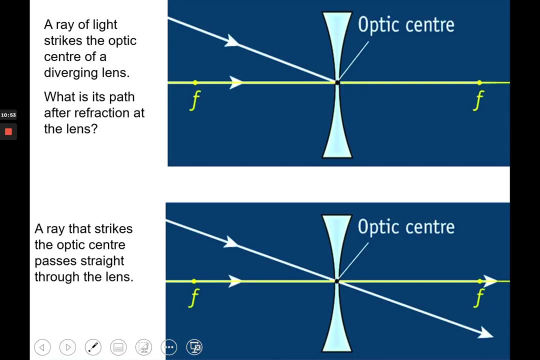 again, our formula for magnification is v over u for our image, distance over our object distance. okay, to see whether it's magnified or diminished up. next we've got our diverging lens, also known as a concave lens. our rules slightly similar, but we need to know the differences. there's some differences between the two, so we're going to 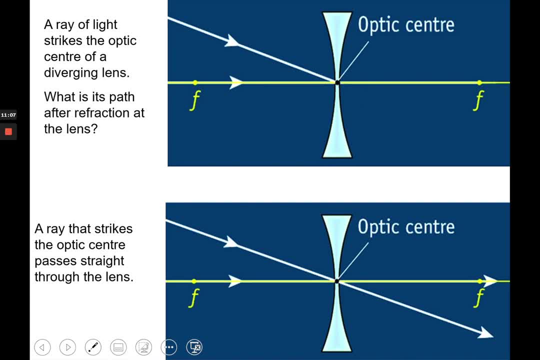 talk about that a little bit later. small differences, guys. they're intricate, so it takes a little bit of time to study these in order to get them correct. the first one, however, is the same: as our converging lens, light ray traveling towards our optic center continues to travel in a straight line on through, okay. 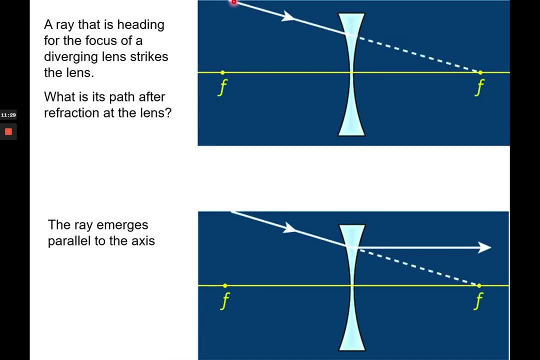 passes straight through. if a light ray is coming in and it looks like it's heading, or it's heading towards the focal length, what happens is it does not head towards the focal length because it's going to refract, it's going to bend, and it bends parallel to the principal axes on the far side of the diverging lens. 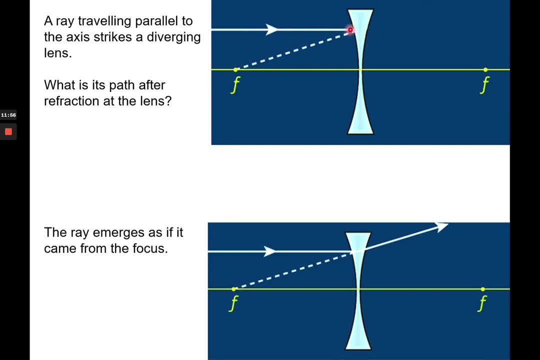 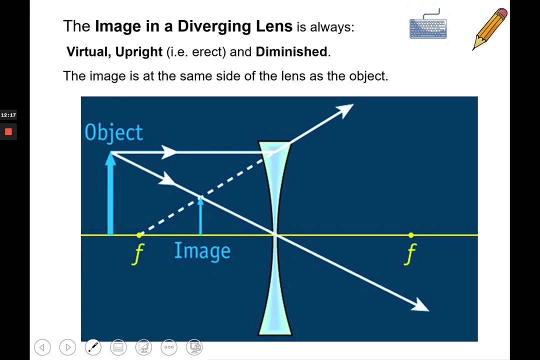 up. next, if it's coming, if we've got a light ray coming in parallel to the principal axes, it will diverge out or spread out as if it's coming from the focal point. okay, so it emerges as if it came from the focal point, and what we can do now is we can combine these rules to see where our image is going to form. 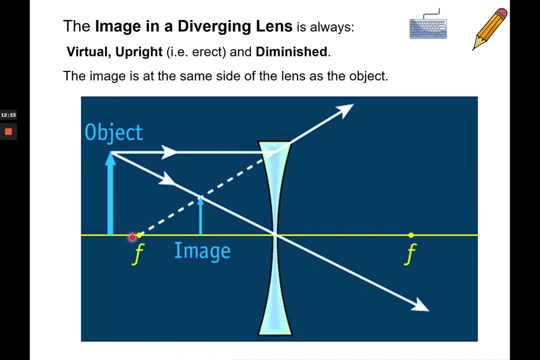 okay, so here we've got our object outside the focal point. our first light ray. all right, there we go. our first light ray parallel to the principal axis and it's coming diverging out as if it came from the focal point. our second light ray, heading straight for the optic center, and it passes straight through. now let's have a look. 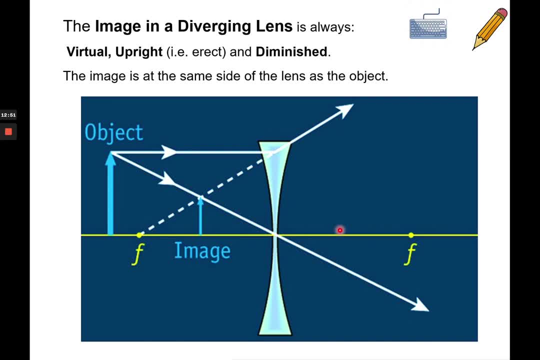 on the right hand side of our lens. these two light rays are diverging. they're never going to meet, so therefore we have to trace them backwards, and we find here. when we trace them backwards, is where they intersect, and here is where our image is going to form in a diverging lens. 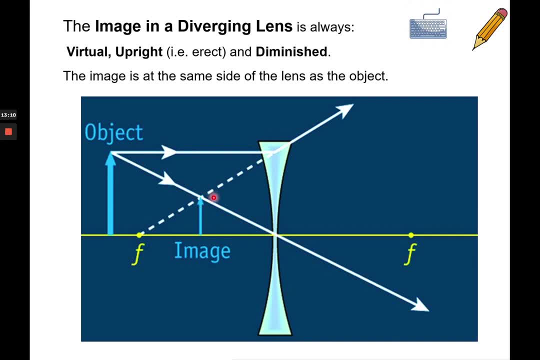 the image is always virtual, which means it's always going. you're always going to have to trace your light rays backwards. it's always going to be upright. we can see it's on the same side of the principal axis as our object. it's above the principle axis and it's diminished. 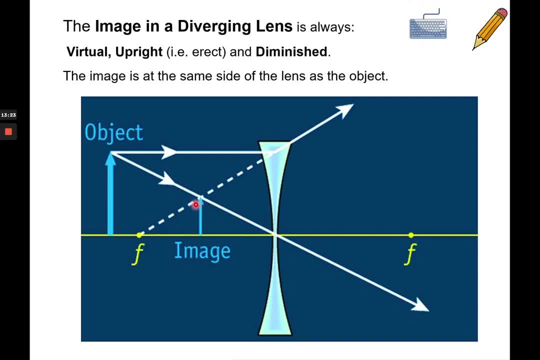 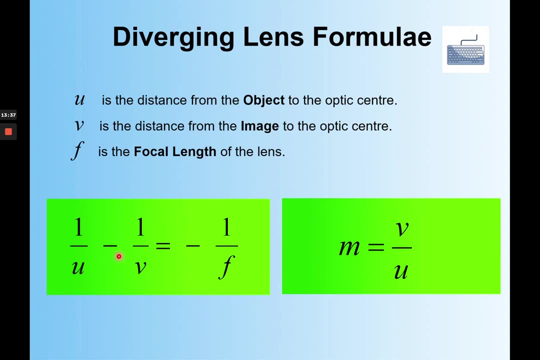 we can see, it's much smaller. okay, the image will always be on the same side of the lens as the object. it will never appear on the right hand side of our lens. okay, so going to be a virtual image. we've got a minus here in front of our v for our image and we've got a 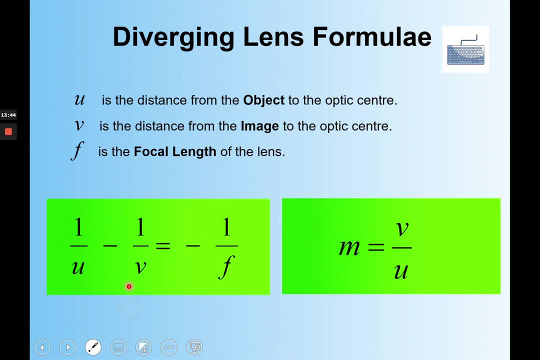 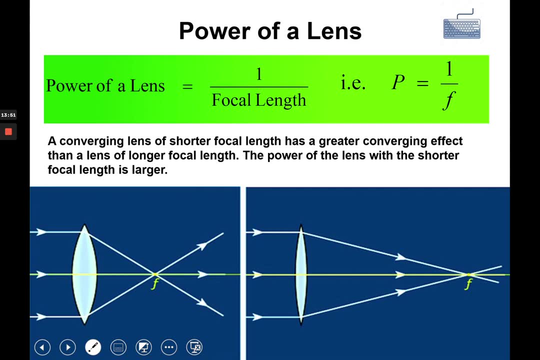 minus in front of our focal length as well. up next, guys, we're going to have a look at the power of a lens, simply given, power is given by a capital, p, and it's equals to one over the focal length. okay, now things to note: that focal length, if you're given that, uh, if you're given that measurement. 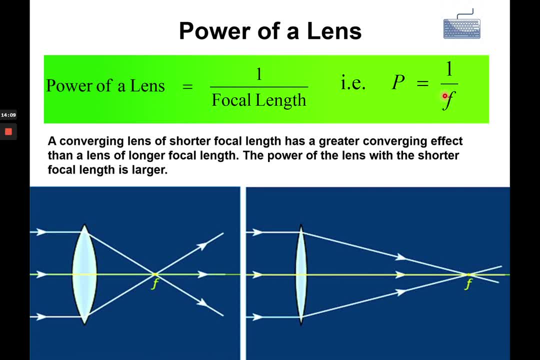 in centimeters, always converted into meters. so if you're given 20 centimeters converted into 0.2 meters- and let's have a look here- we can see the shorter the focal length. hopefully the more powerful the lens is. here we've got a longer focal length and the lens is not as powerful. 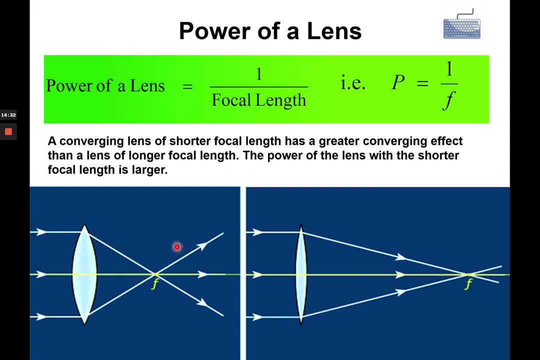 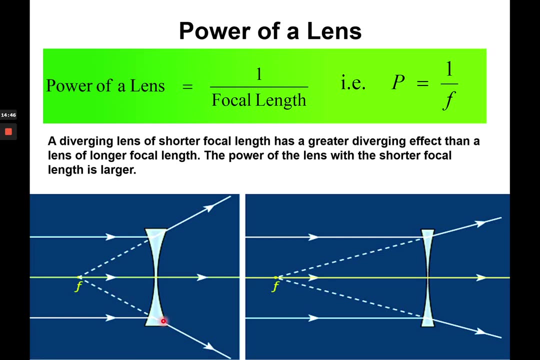 whereas on the diagram on the left we can see there's a huge amount of um, there's a huge amount of refraction occurring here. so shorter the focal length, greater the power. again, in this case, the shorter the focal length, the greater the ability to diverge that light ray or those light rays. 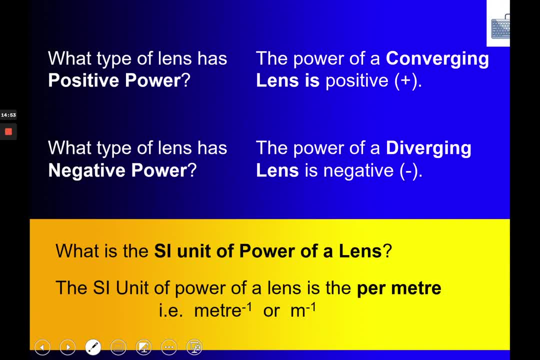 so we said that the SI unit for a power of a lens is per meter, so we always need to ensure that our focal length is given in meters, not in centimeters. a converging lens has a positive power, while a diverging lens has a negative power. 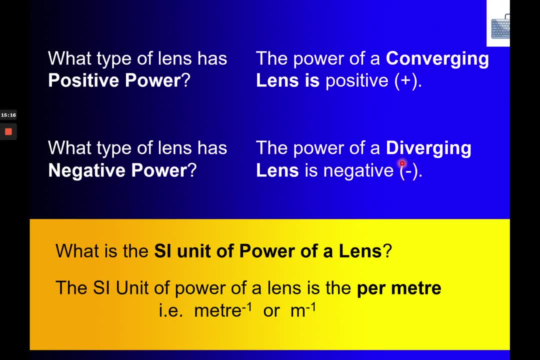 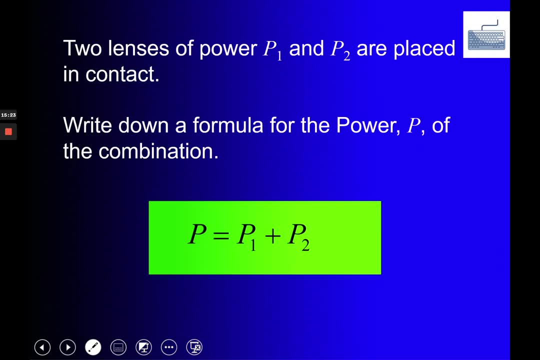 okay. so we need to use a negative sign when talking about a diverging lens. if you two lenses combined, the total power is equals to the power of the first lens plus the power of the second lens. so we need to use a negative sign when talking about a diverging lens. 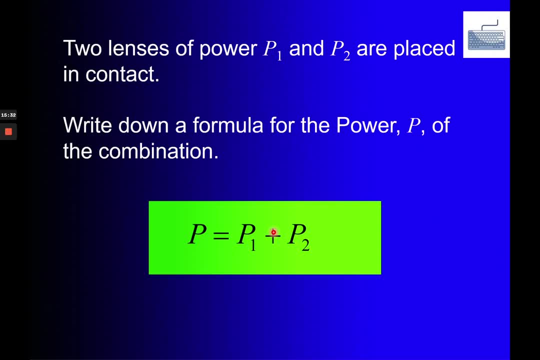 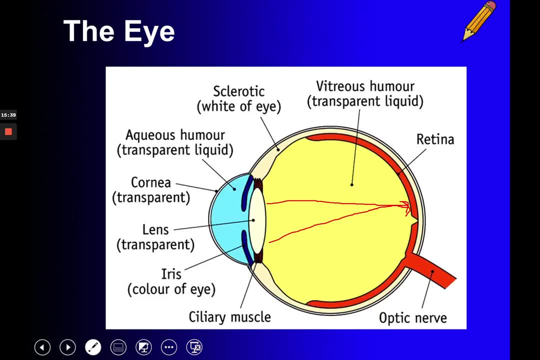 now, if you put a diverging lens in there, well then you need to subtract one from the other. okay, excuse me a second. so our eye acts as a lens and we can see we've got a lens, fine, here in the middle of our eye, and the reason for that is that we can make a difference between the two lenses, so we can 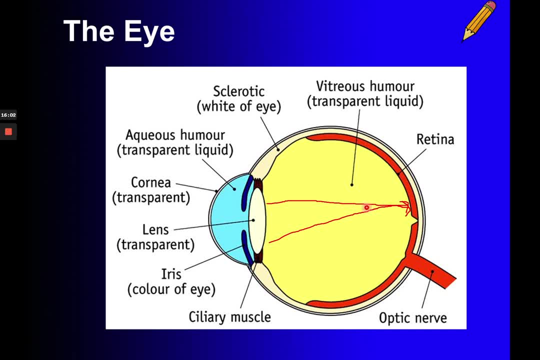 bend light and get that light to bend and focus on the retina, which is like the screen at the back of our eye. okay, so, depending on whether we're in a very bright room or a very dark room, these ciliary muscles above and below the lens will either contract or extend to change the shape. 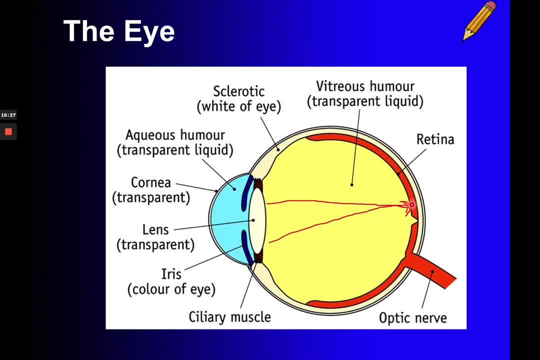 of our lens so that light always gets focused onto the retina and the eye, so that we can see that light is at the back of our eye. then our retina is connected to an optic nerve which takes these signals to our brain and our brain converts them into the images that we see every day. 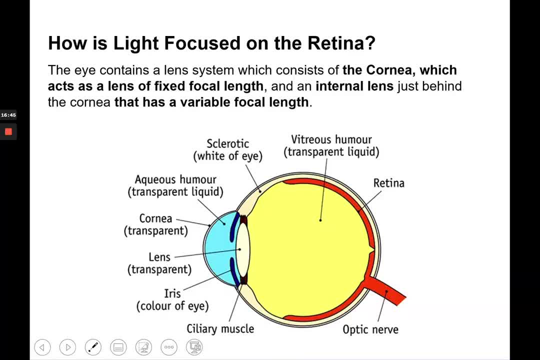 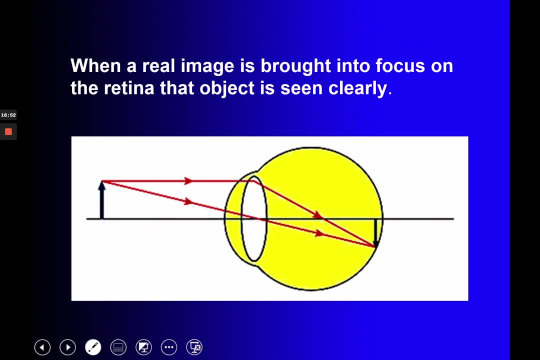 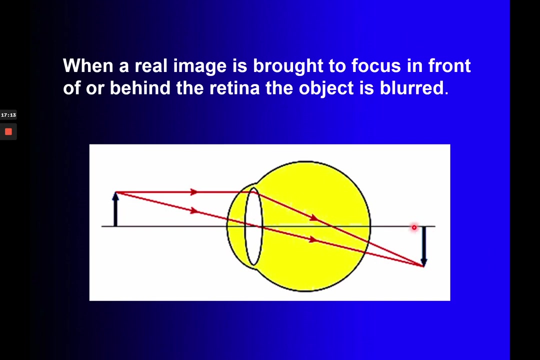 okay, which is pretty incredible. when a real image is brought into focus on the retina, the object can be seen clearly like a in this diagram. so we've got our lens in the middle of our eye and we can see our image is forming directly on the retina, and that's great. however, if the object is brought into focus behind, 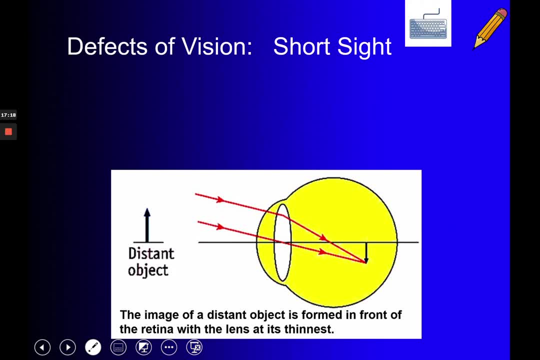 the retina. well then, the image will appear blurry. likewise, if it's brought in to focus below, before the retina, like in this case, our retina is the back screen, the screen at the back of our eye. it's brought into focus before the retina, so it's not going to be a blurring image and we can see. our image is. 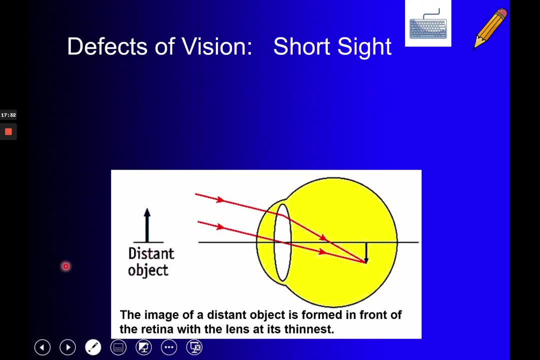 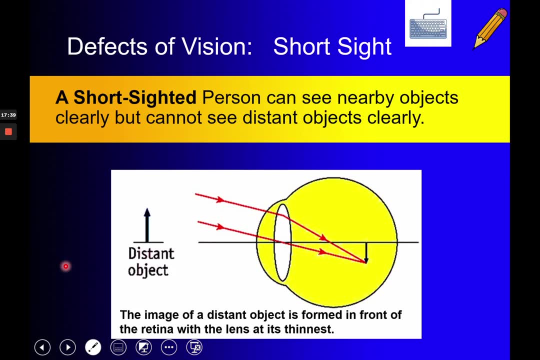 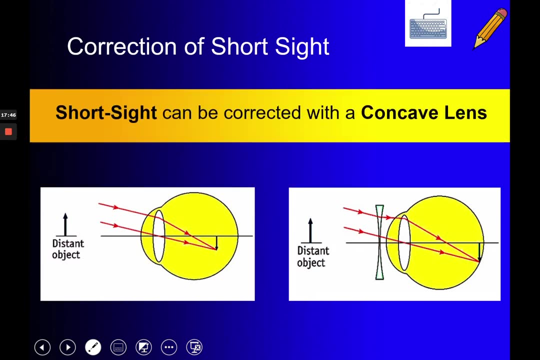 that again, the image will appear blurry. and in this case, someone who is short-sighted can see nearby objects but cannot see distant objects clearly, and the correction for short sightedness is to use a diverging lens. and what happens here? if we have a look at the diagram on: 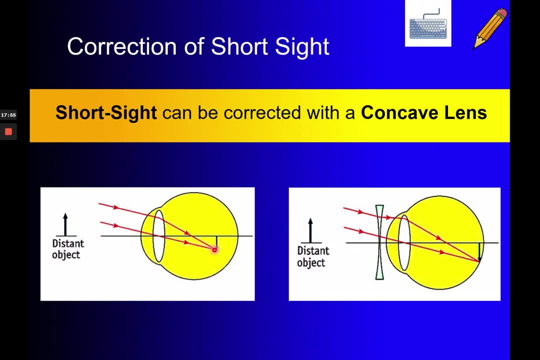 the left, first up, we can see that the image is appearing in the center of the eye, while it should be appearing at the retina at the back of the eye. so what we can do is take a diverging lens which actually spreads out the light rays ever so much and therefore, when they're spread out by the time, 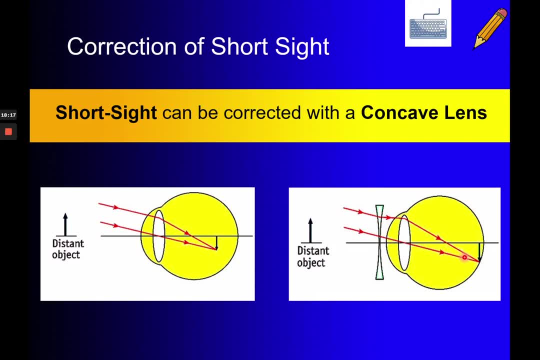 that our at the lens of our eye gets a hold of those two light rays, it will then connect with the yellows. so when the red light is connected to the yellow lens, it will then connect to the orange lens and the green lens, and then it will connect to the blue lens. so 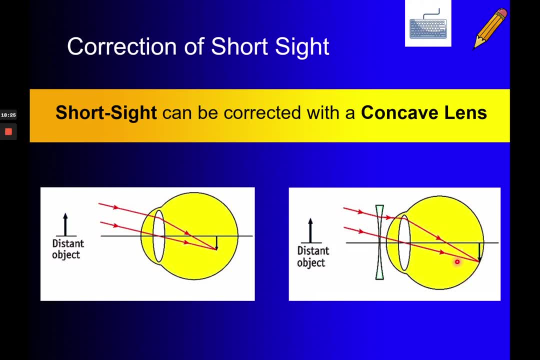 the red lens and the blue lens will connect to the blue lens and the red lens and then it will then converge them at the back of the eye, at the retina, where we want the image or where we want the light rays to intersect, and now we've got a clear image forming, which is brilliant. 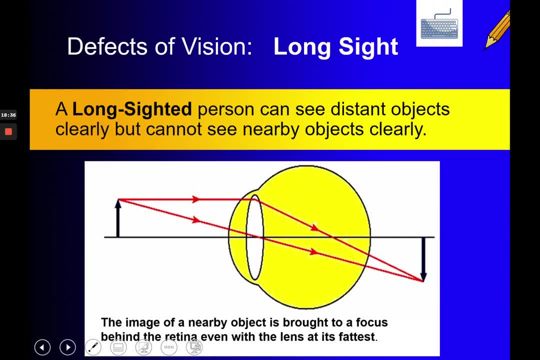 someone who's long-sighted can see distant objects clearly but cannot see nearby objects. so we can see here: this is long-sighted, because while we want our image forming on the retina, we can see, the image isn't forming until behind the eye, which is no good. so what we can do, we can. 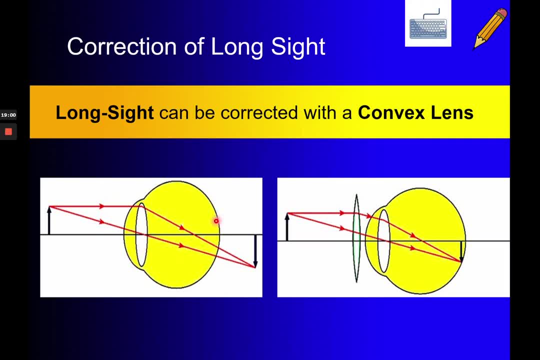 see the lens. our lens is not strong enough to get the light rays to focus on our retina, so what we do is we put another converging lens or convex lens in front of our eye and this focuses it. this focuses the light ray, and then the lens of our eye focuses the light rays one more time.